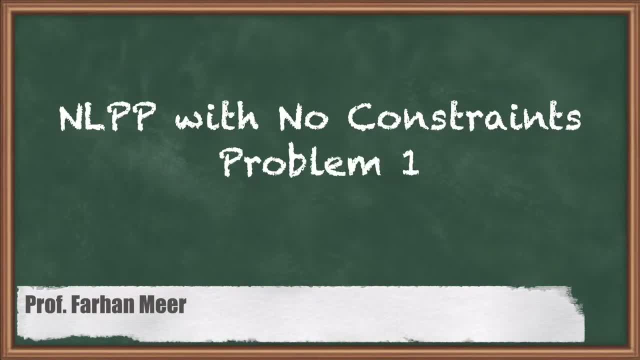 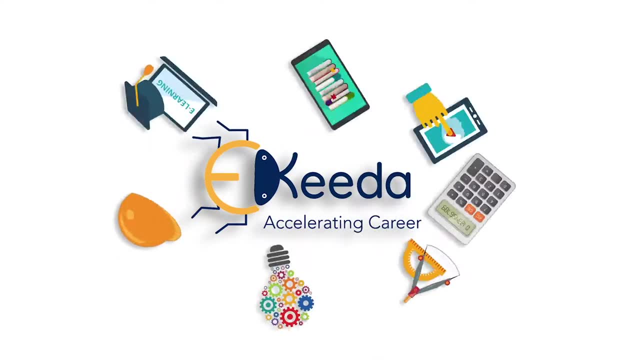 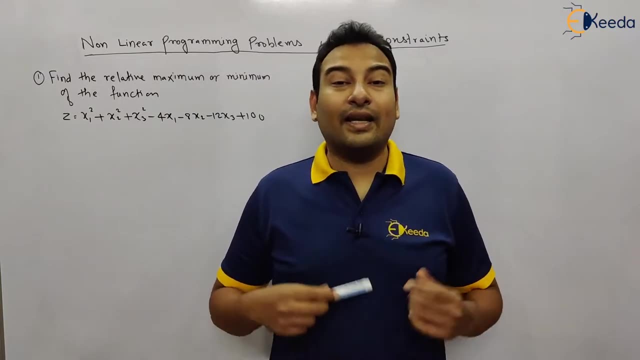 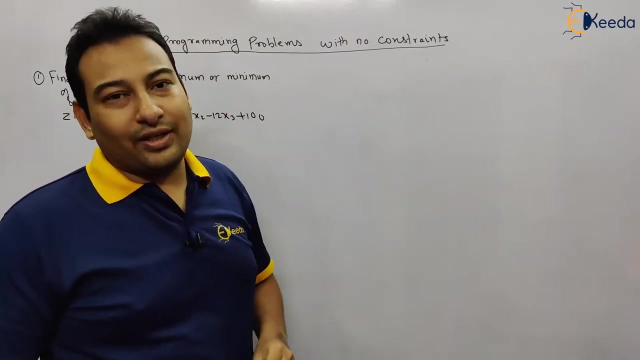 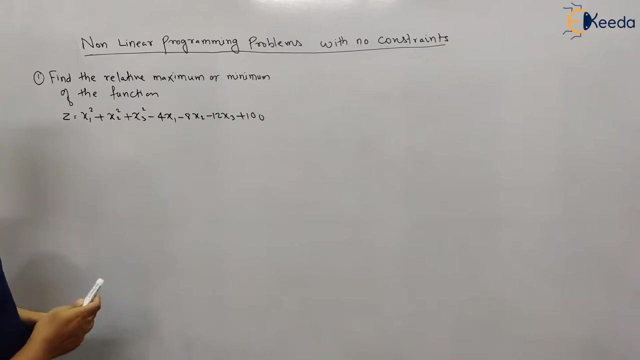 Hello friends, in this video we'll be discussing nonlinear programming- problems with no constraint, problem number one. Welcome back, students. now we are starting with the next topic, that is, NLPP, and the first type of problems are nonlinear programming problems with no constraint. So this is the given problem. we need to find its relative maxima or minima, and this is called your objective. 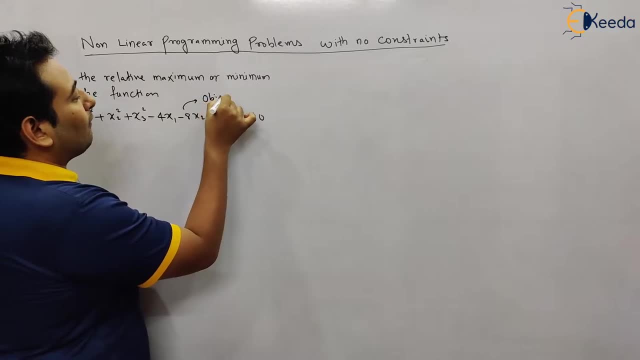 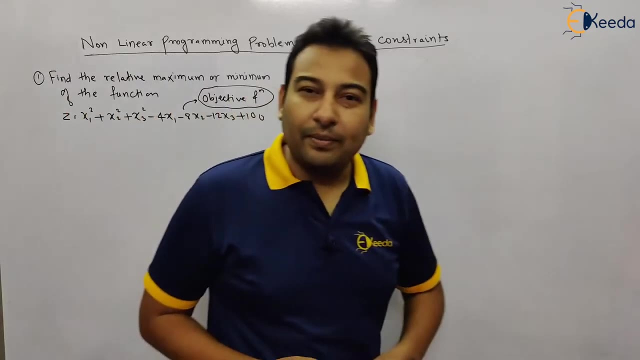 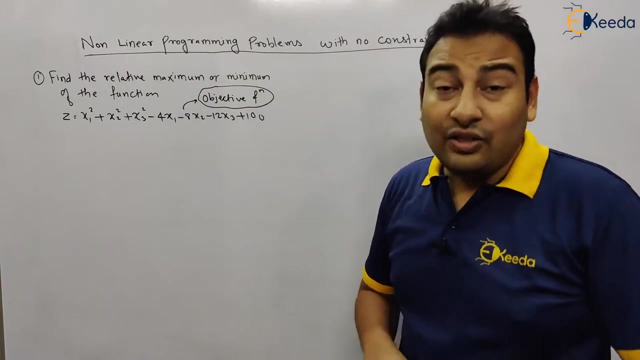 function and in the given problem there is no constraint, no restriction given. So we need to find a relative maxima or minima of this, of this function and, as the name suggests, nonlinear programming problems. there is one more chapter, linear programming problems. So what is the? 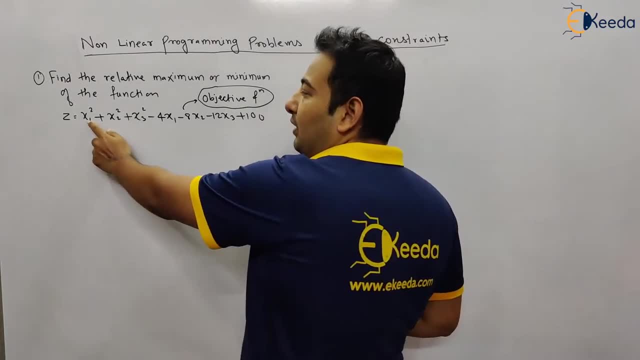 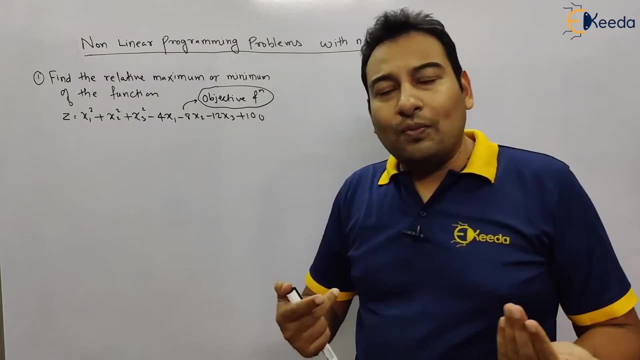 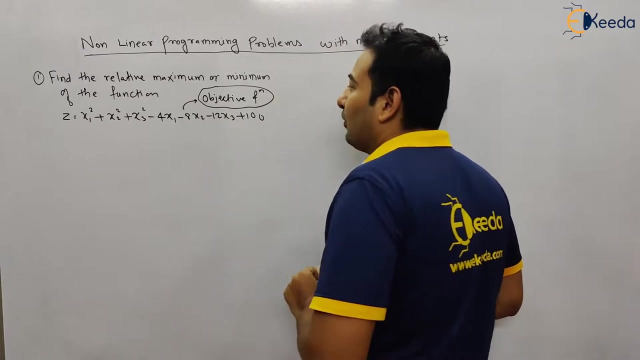 difference between linear and nonlinear. See the terms, see this: Squares, squares. this indicate nonlinear. So this square or cube, it indicates nonlinear programming problems and our aim is to find the relative maxima or minima of this particular function and there are no constraint given. 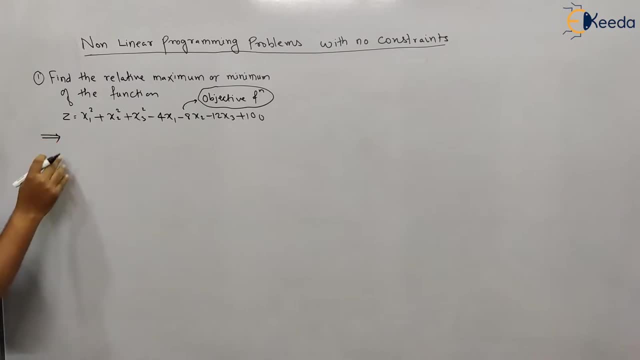 So let us start with the solution. First of all, let's assume this function as x1, x2, x3.. Let me assume this z as function of x1, x2 and x3. that is equal to same function. i am copying: there is a concept of hashen matrix. first of all, let us discuss that hashen matrix. see the way i. 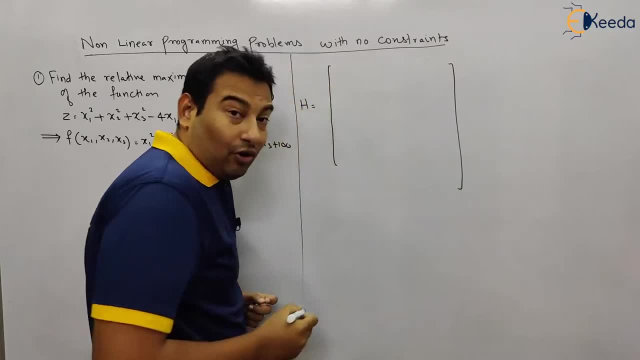 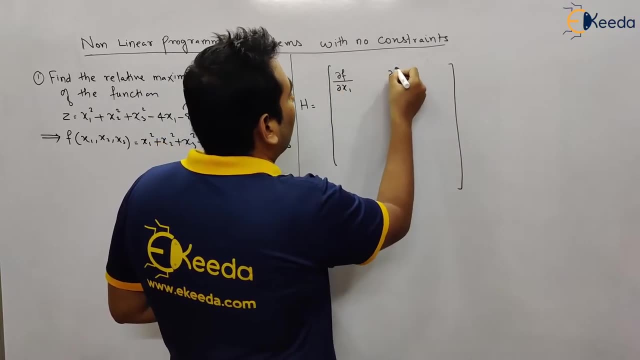 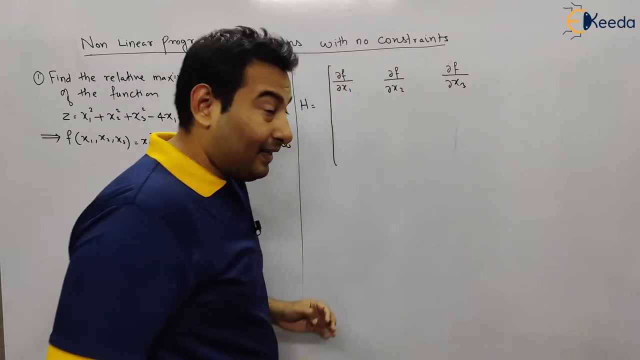 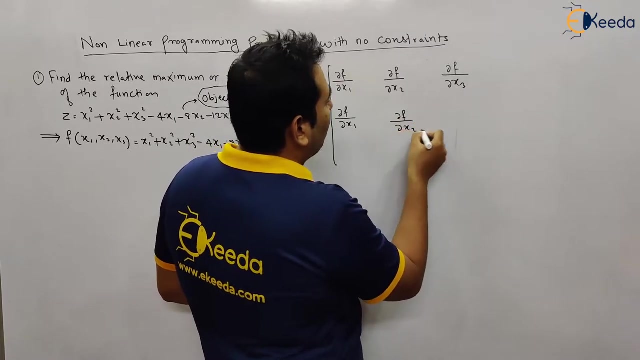 am writing this matrix, i am forming this matrix. this is very important. first of all, i am going to write it down here: dou f upon dou x1. see the way i am writing: dou f upon dou x2 and dou f upon dou x3. next, repeat this thing: dou f upon dou x1. again, dou f upon dou x2. i will tell you what is. 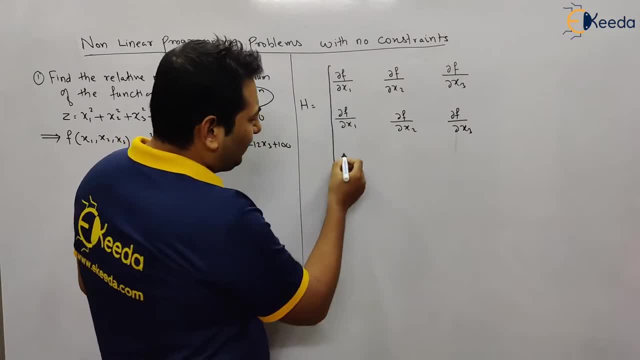 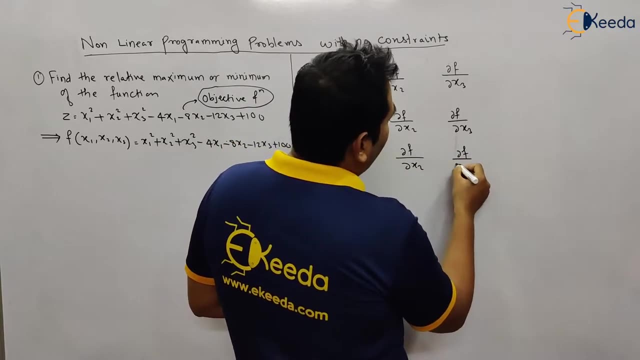 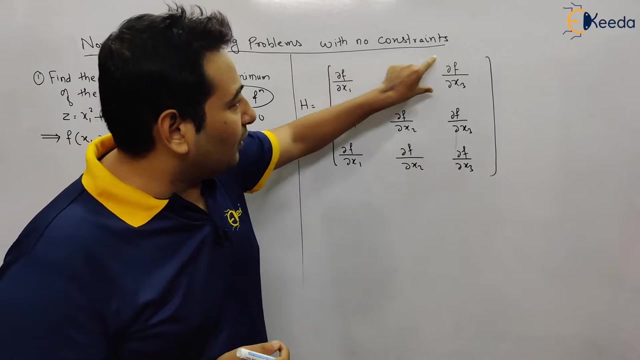 the use of this matrix. first of all, let us see how to form this matrix: dou f upon dou x1, dou f upon dou x2 and dou f upon dou x3. so this is your hessian matrix. now for the first row we going to differentiate with: 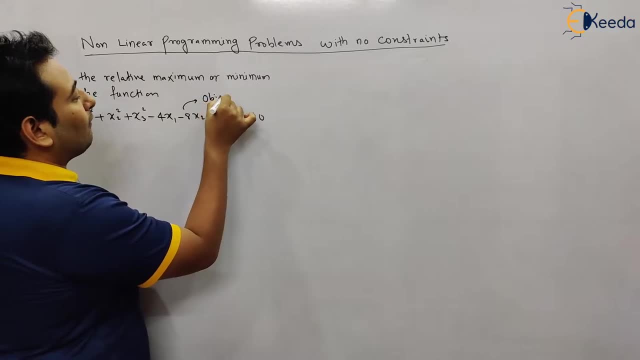 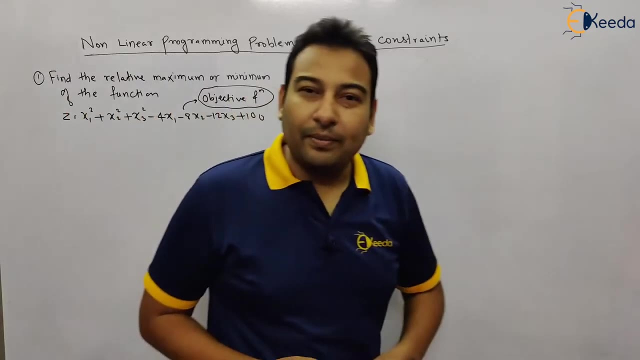 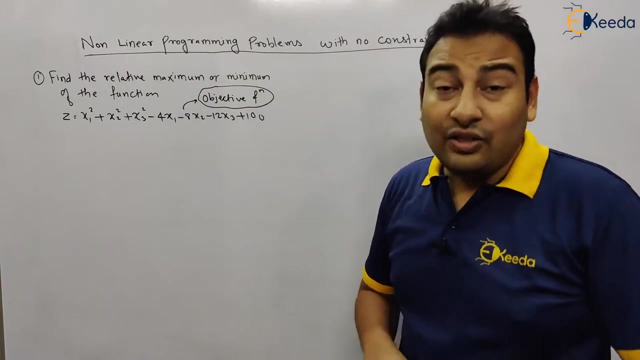 function and in the given problem there is no constraint, no restriction given. So we need to find a relative maxima or minima of this, of this function and, as the name suggests, nonlinear programming problems. there is one more chapter, linear programming problems. So what is the? 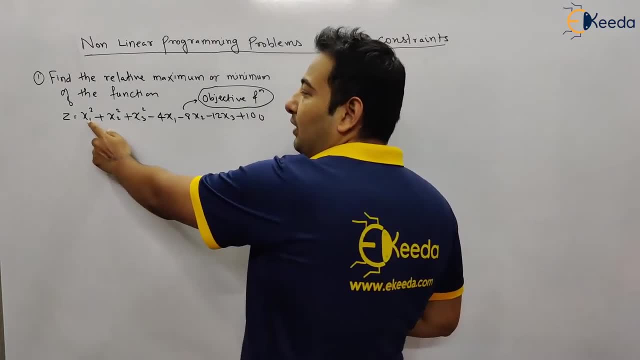 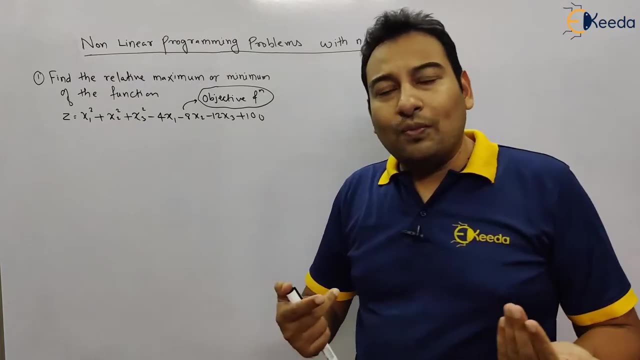 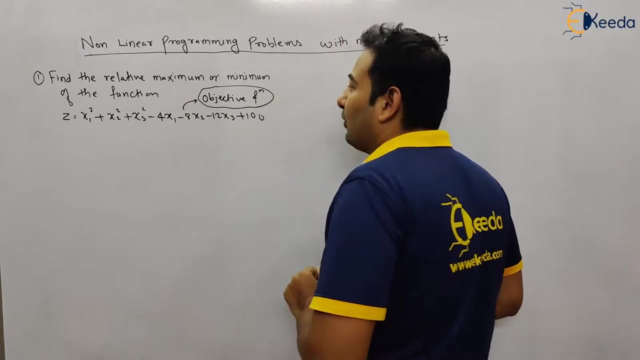 difference between linear and nonlinear. See the terms. see this square- square- this indicate nonlinear. So this square, or cube, it indicates nonlinear programming problems and our aim is to find the relative maxima or minima of this particular function and there are no constraint given. So let us start. 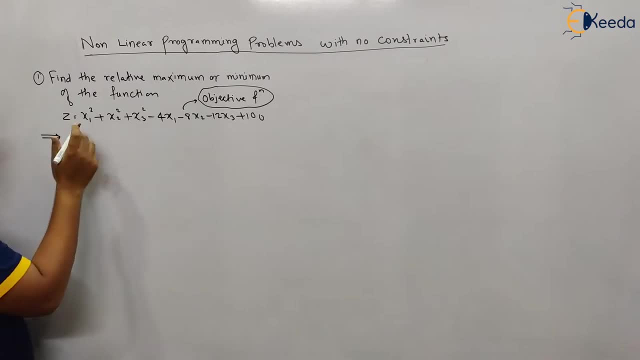 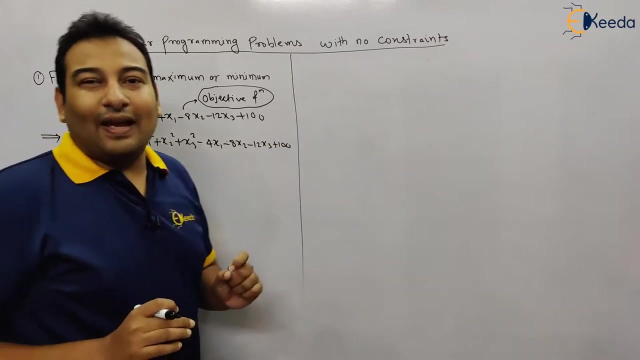 with the solution. First of all, let us assume this function as X, 1 comma, X, 2 comma, X, 3.. Let me assume this z as function of x1, x2 and x3. that is equal to same function. i am copying: there is a concept of hashen matrix. first of all, let us discuss that hashen matrix. see the way i 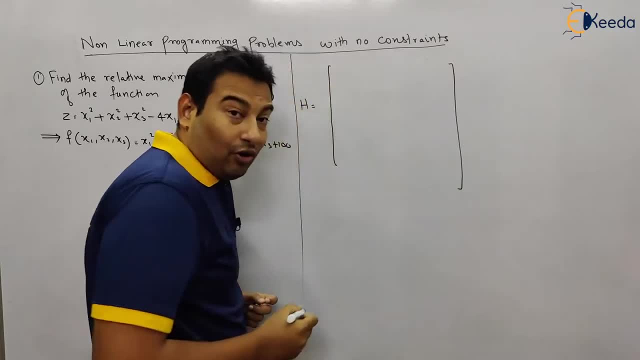 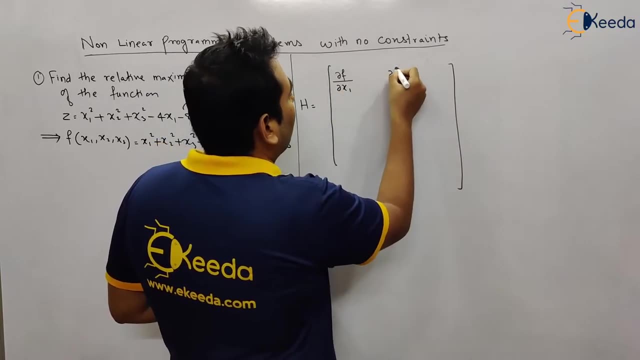 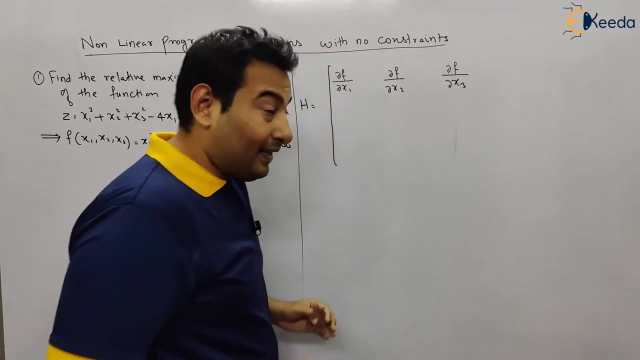 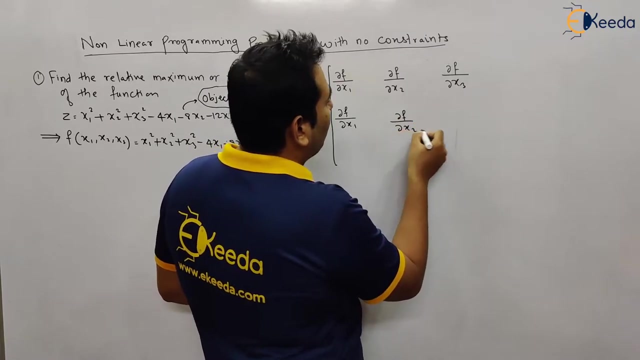 am writing this matrix, i am forming this matrix. this is very important. first of all, i am going to write it down here: dou f upon dou x1. see the way i am writing: dou f upon dou x2 and dou f upon dou x3. next, repeat this thing: dou f upon dou x1. again, dou f upon dou x2. i will tell you what is. 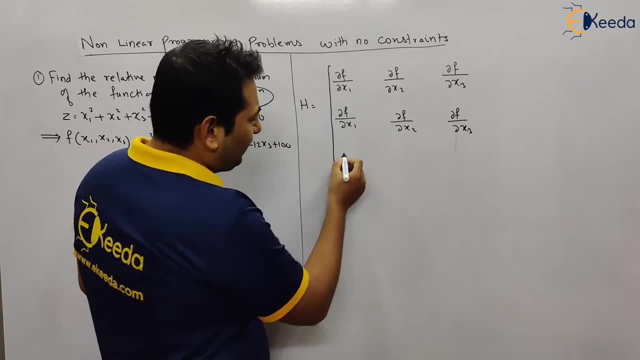 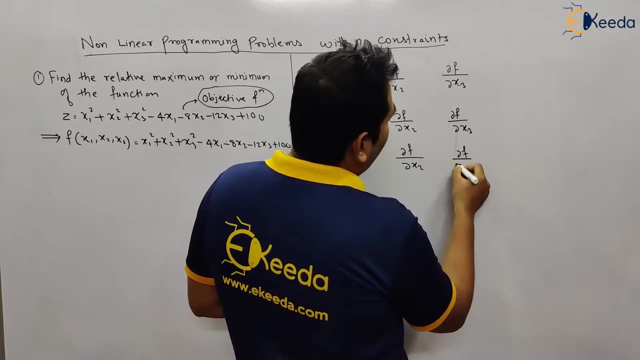 the use of this matrix. first of all, let us see how to form this matrix: dou f upon dou x1, dou f upon dou x2 and dou f upon dou x2 and dou f upon dou x1 and dou f upon dou x2. and dou f upon dou x1 and dou f upon dou x2. 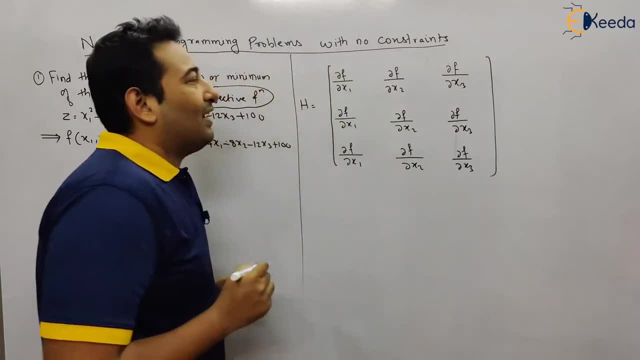 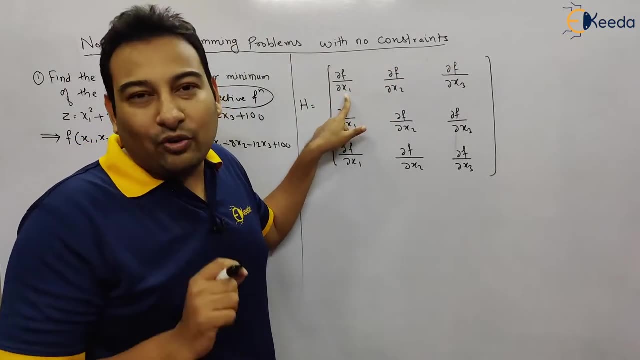 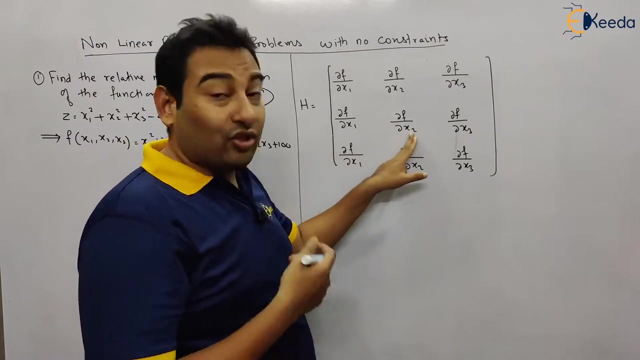 dou f upon dou x3. so this is your hashen matrix. now, for the first row, we going to differentiate with respect to x partially, so let us differentiate all the terms with respect to x. second row, i am going to differentiate with respect to x2 and for third row, i am going to differentiate with: 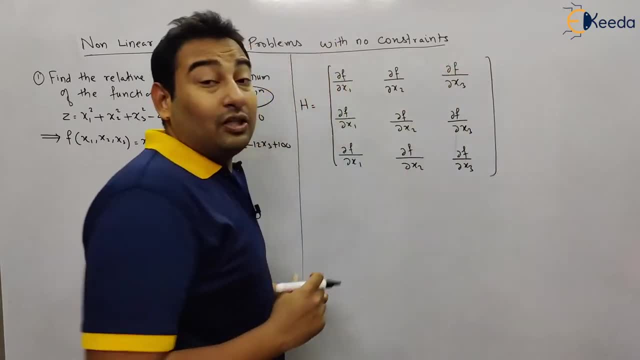 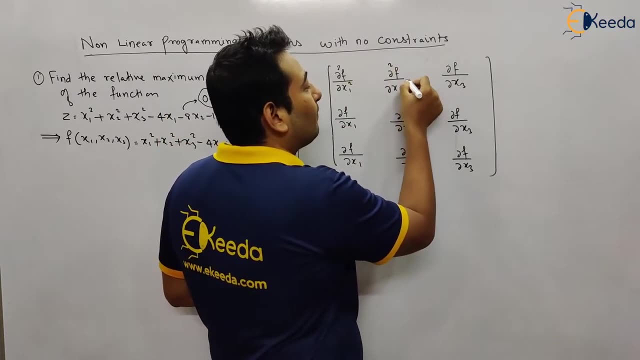 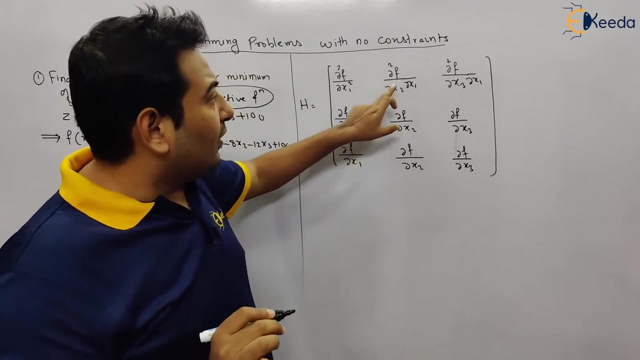 respect to x3. so if i differentiate the first row with respect to x1, this will be double derivative. with respect to x1, this will be x2- x1 and this will be x3- x1. let me tell you first of all, note this point- dou square f upon dou x2, x1. 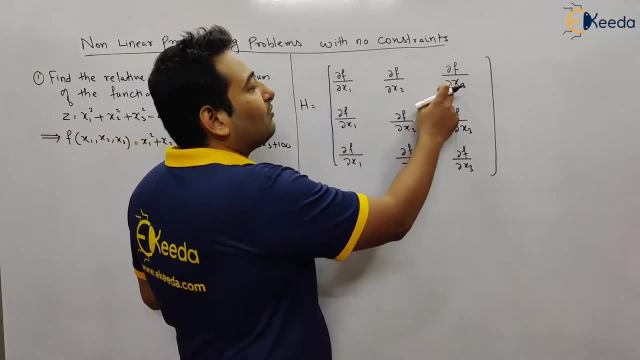 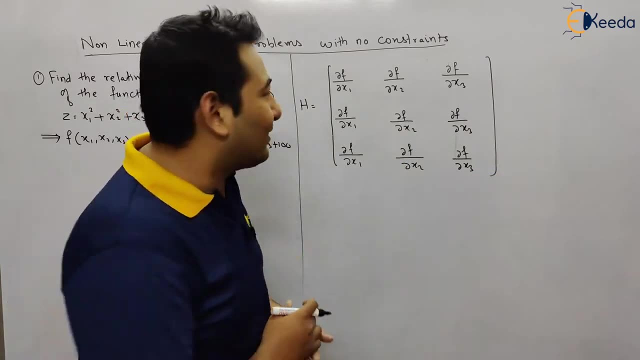 respect to x partially. so let us differentiate all the terms with respect to x. second row, i'm going to differentiate with respect to x2 and for third row, i'm going to differentiate with respect to x3. so if i differentiate the first row with respect to x1, this will be double derivative. 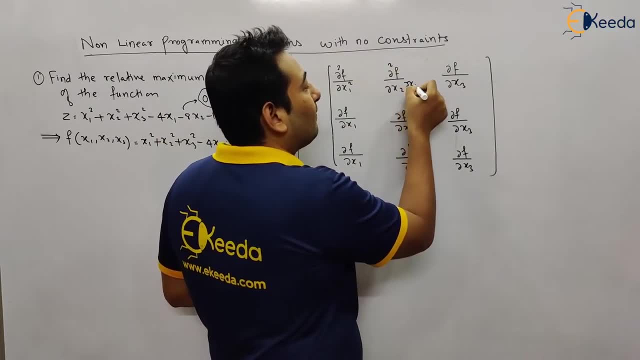 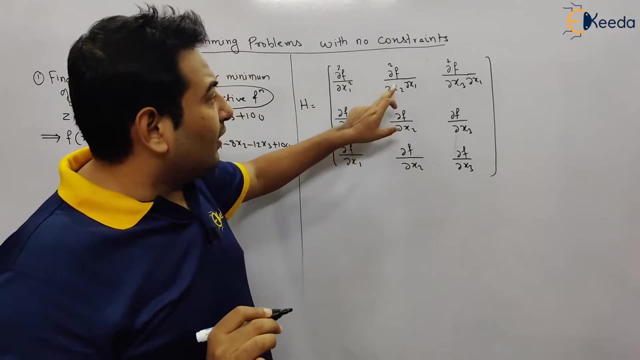 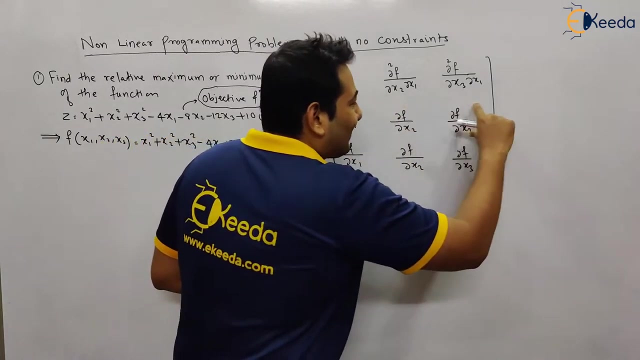 with respect to x1, this will be x2- x1 and this will be x3- x1. let me tell you first of all, note this point: dou square f upon dou x2, x1 or x1- x2, both are same, okay, so let us differentiate the. 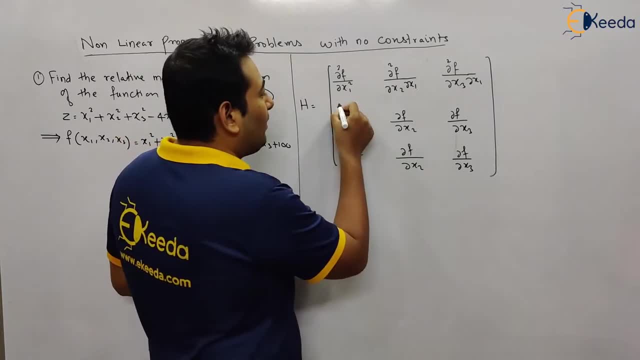 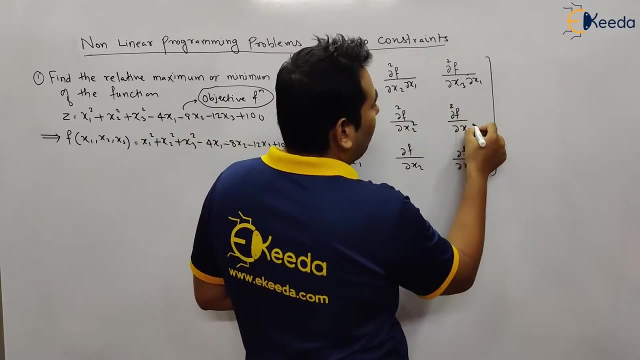 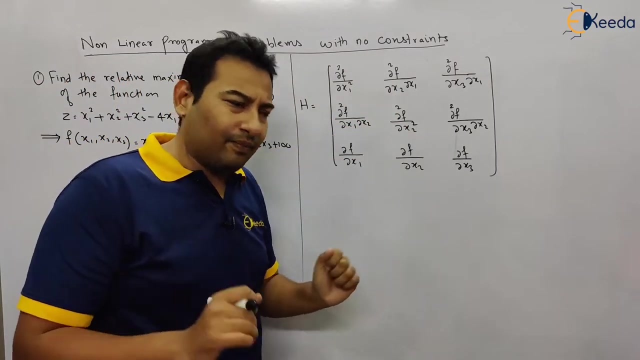 second row with x2. so it will be x2 with x2. then it will be double differentiation. with x2, x2 will come here. these two terms are same, so x2, x1 or x1, x2 doesn't matter, they are same. okay, this is the property of. 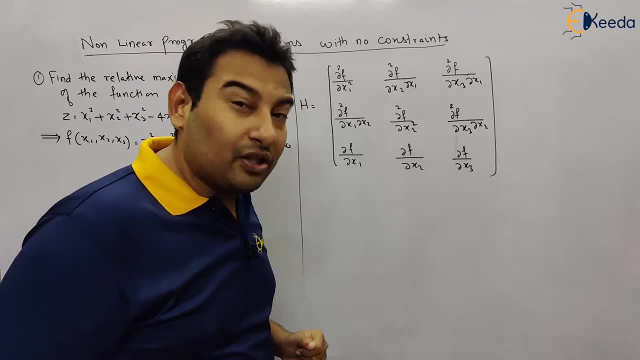 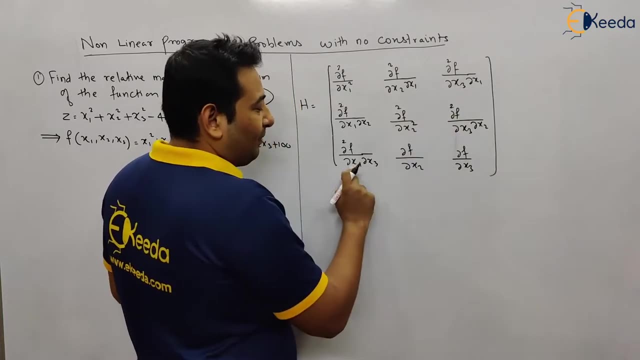 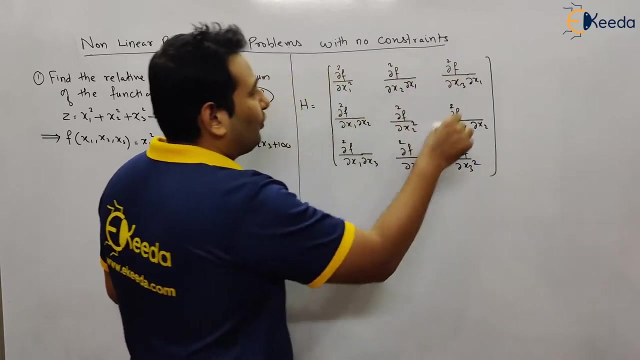 partial differentiation. next, the last row: we are going to differentiate with respect to x3, so this will be x3. again, these two terms will be same: x1, x3, x3, x1 doesn't matter, they are same. and finally, so this is your hessian matrix. 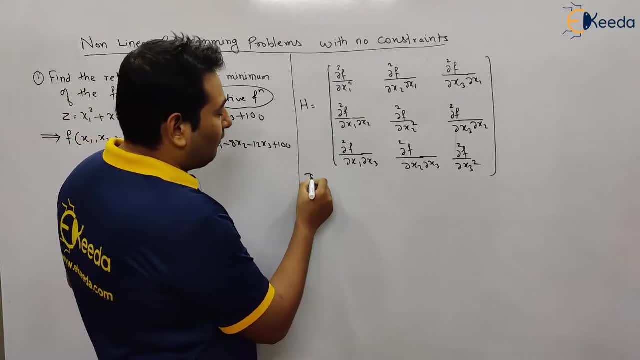 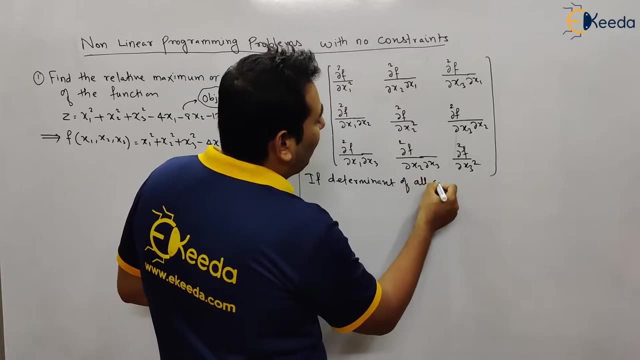 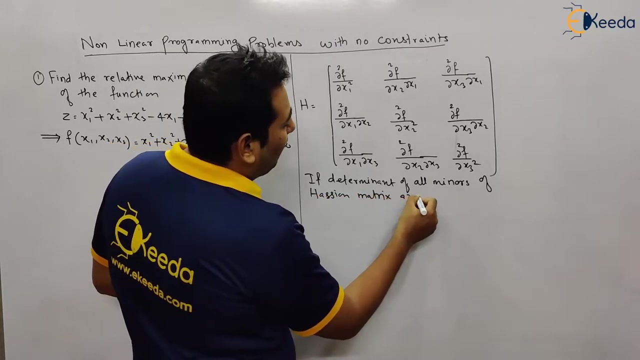 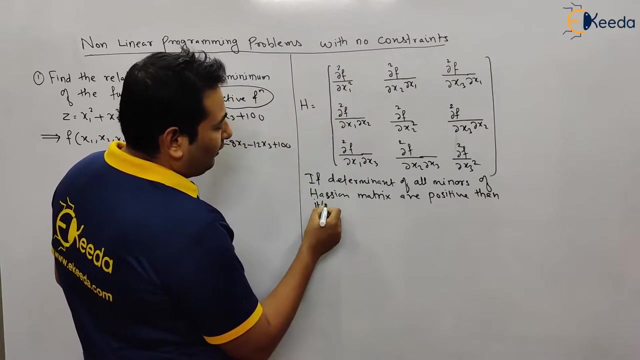 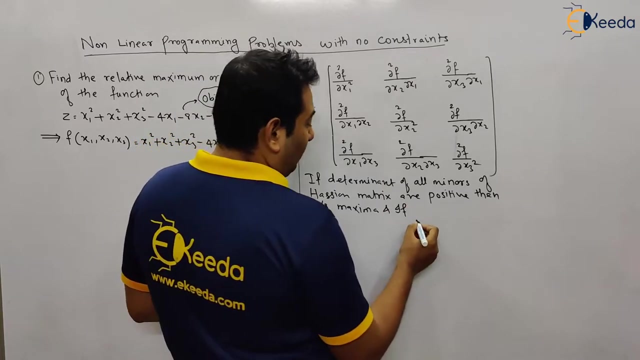 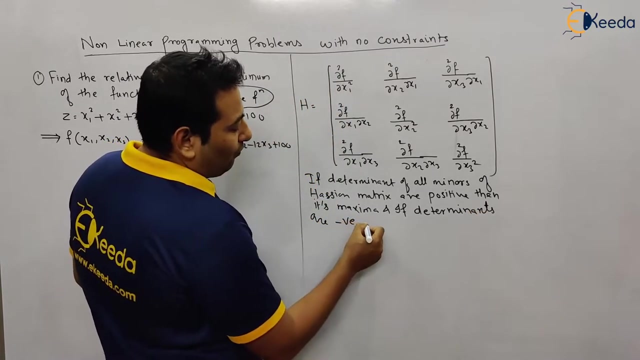 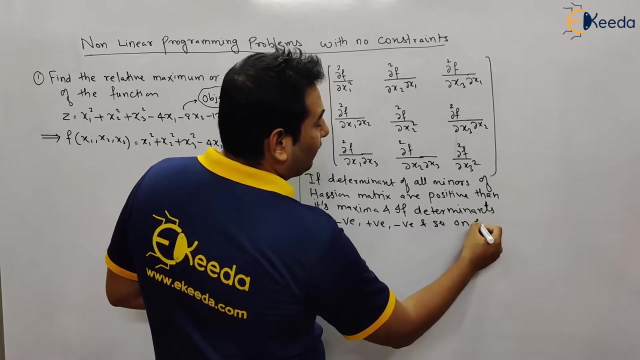 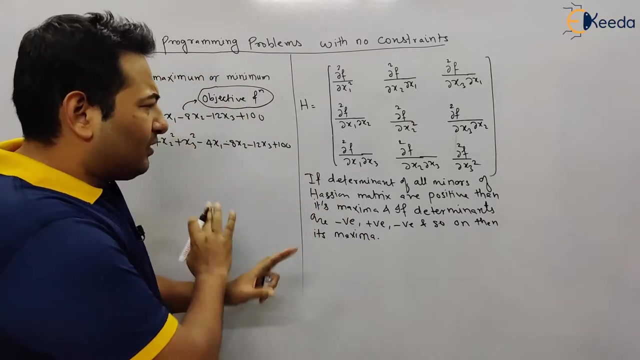 if very important point, if determinant of all minors of hessian matrix are positive, then its maxima. and if this point is very important and if determinants are negative, positive, negative and so on- that means alternate negative, positive and so on- then its maxima. what are the? these things we are going to discuss later on. as of now, just remember this. 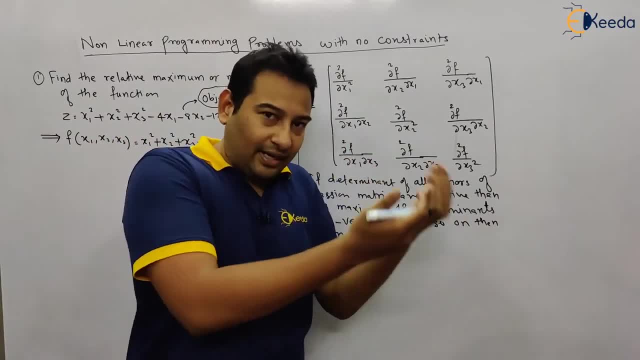 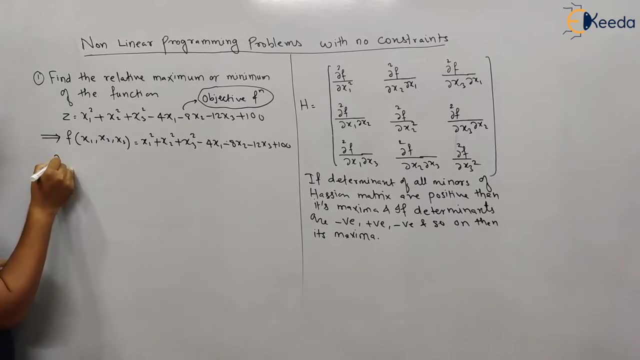 hessian matrix. i hope this is clear. how to form the hessian matrix. let's come back to the original problem. this is my f. so first of all, i'm i'm going to differentiate this hessian matrix with respect to x1, and then i'm going to differentiate this f with respect to x1. 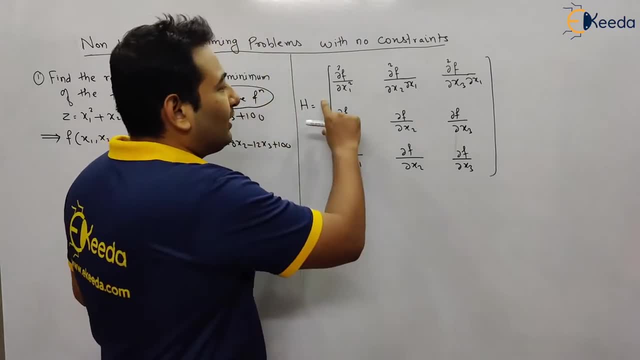 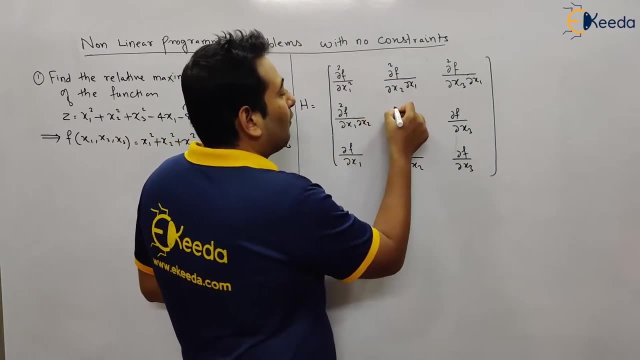 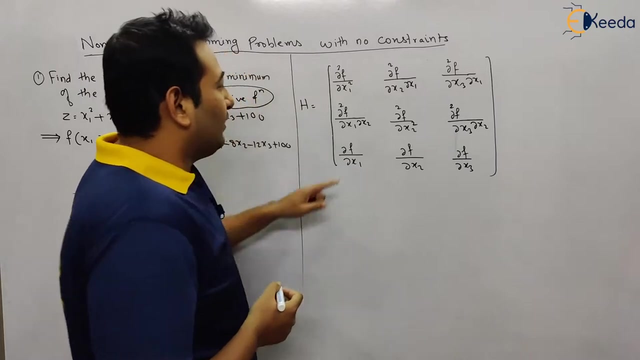 or x1- x2. both are same, okay. so let us differentiate the second row with x2, so it will be x2 with x2. then it will be double differentiation. with x2, x2 will come here. these two terms are same, so x2- x1. 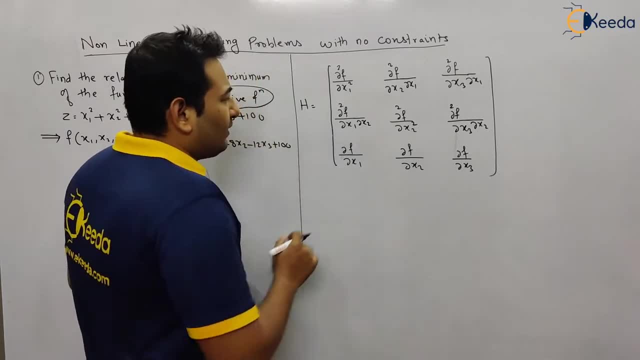 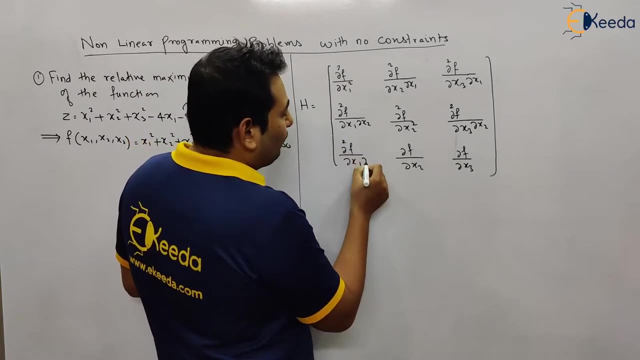 or x1, x2, doesn't matter, they are same. okay, this is the property of partial differentiation. next, the last row. we are going to differentiate with respect to x3, so this will be x3. again, these two terms will be same: x1, x3, x3, x1. doesn't matter, they are same. 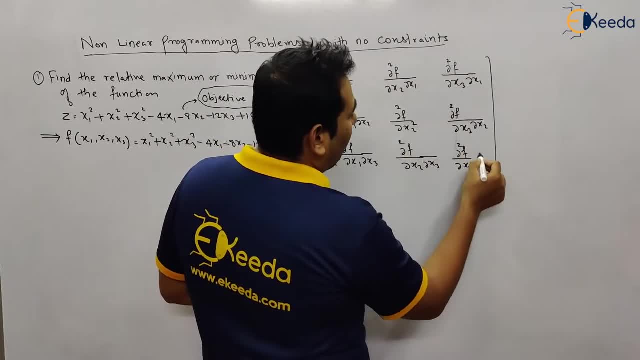 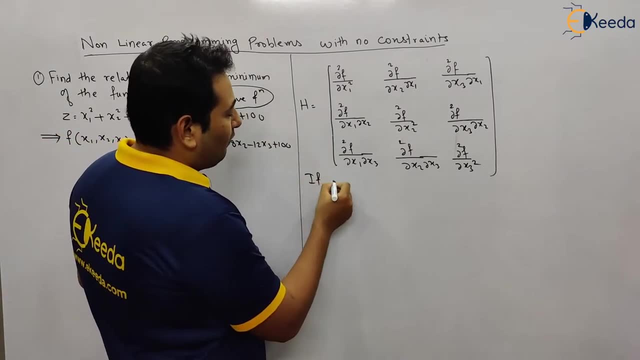 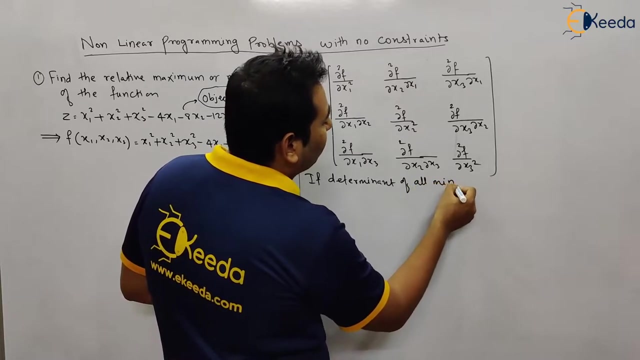 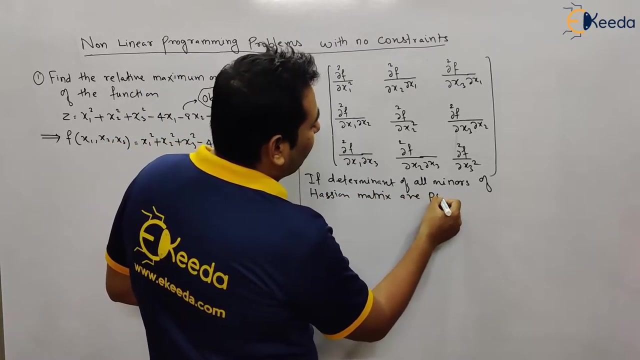 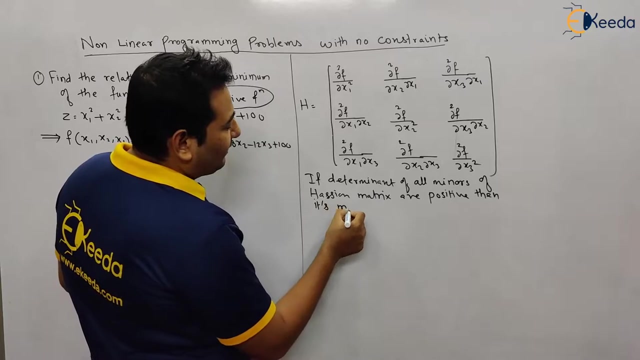 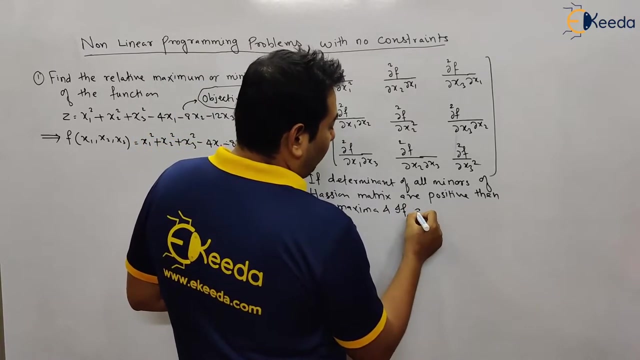 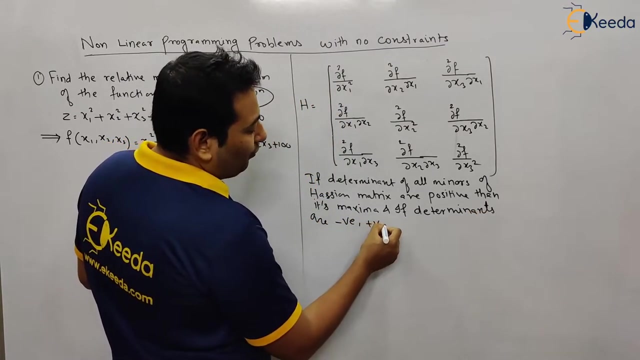 and finally, so this is your hashen matrix. if- very important point, if determinant of all minors of hashen matrix are positive, then its maxima. and if this point is very important and if determinants are positive, then its maxima is x2.. that means we just operate, given negative, positive, negative and so on. 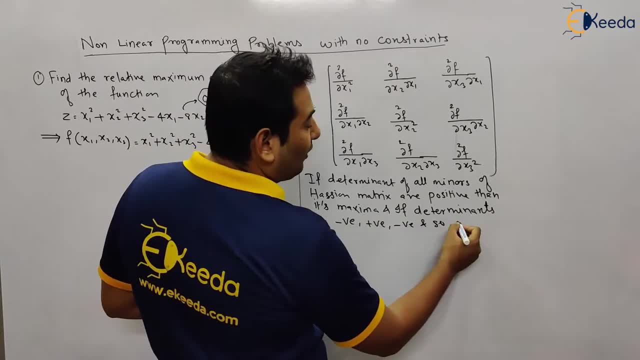 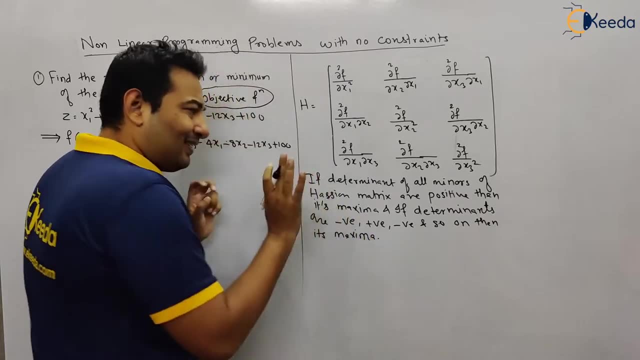 that means alternate negative, positive and so on. then its maxima. what are the things we are going to discuss later on, as of know? just remember this hashen matrix. i hope this is clear. how to form the hashen matrix. let's come back to the original. 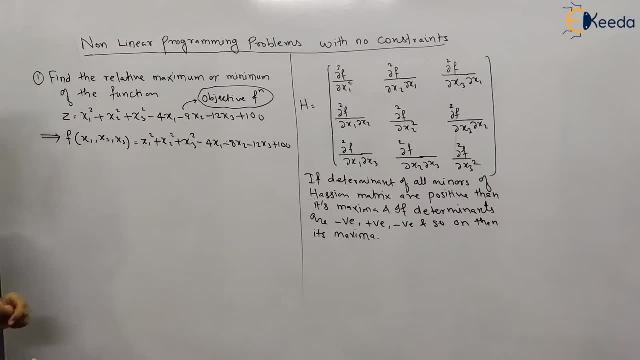 to the original problem. this is my F. so first of all, I'm I'm going to differentiate this F with respect to x1, then I'm going to differentiate F with respect to x2 and I'm going to differentiate F with respect to x3. see the procedure. this F is a function of x1, x2, x3. therefore, we gonna 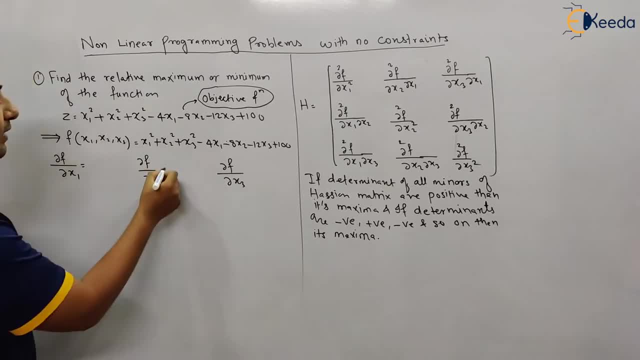 differentiate F with respect to x1, F with respect to x2 and F with respect to x3. let us differentiate with respect to x1, so this will be 2x1. obviously it's a partial derivative concept. when you're differentiating with respect to x1, x2, x3, constant. when you're differentiating with respect to x2. 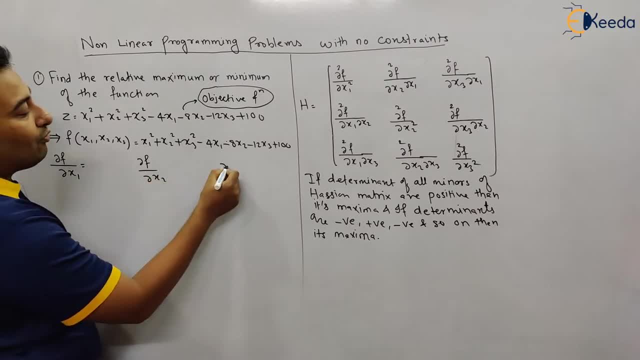 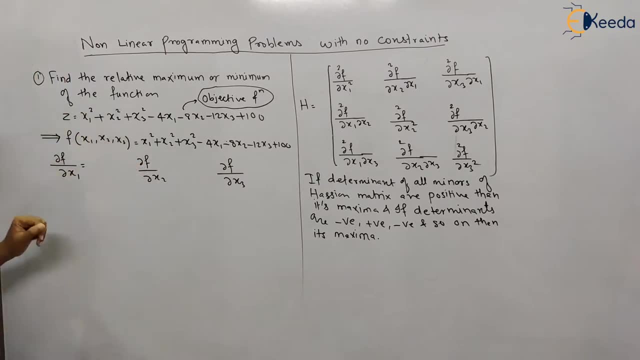 then i'm going to differentiate f with respect to x2 and i'm going to differentiate f with respect to x3. see the procedure. this f is a function of x1, x2, x3. therefore, we're gonna differentiate f with respect to x1, f with respect to x2 and f with respect to x3. let us differentiate with respect to x1. 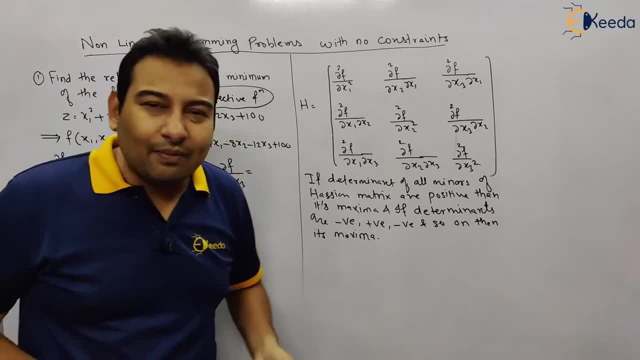 so this will be 2x1. obviously it's a partial derivative concept. when you're differentiating in respect to x1, x2, x3, constant, when you're differentiating with respect to x1, x2, x3, constant, we are disqualifying x2 there. 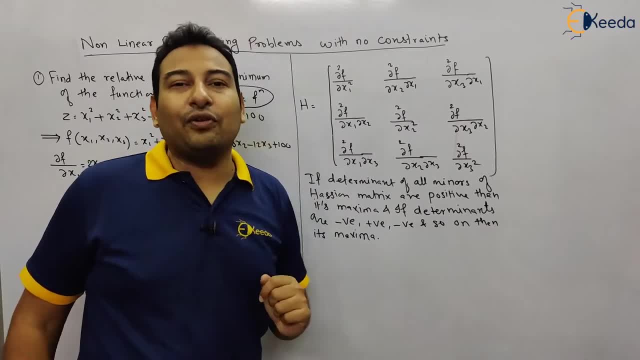 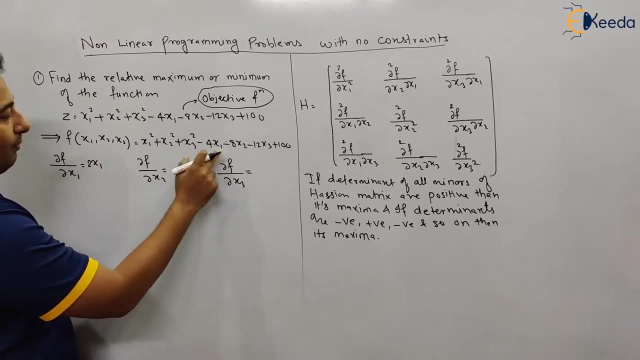 you're differentiating with respect to x2, x1, x3- constant. and when you're differentiating with respect to x3, x1, x2- constant. this is 2x1. this is constant: 0, 0 minus 4 because with respect to x1. 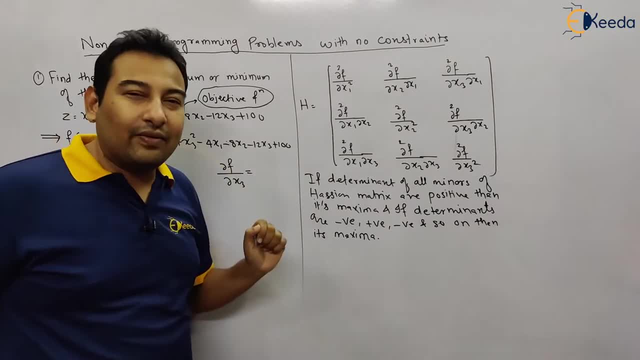 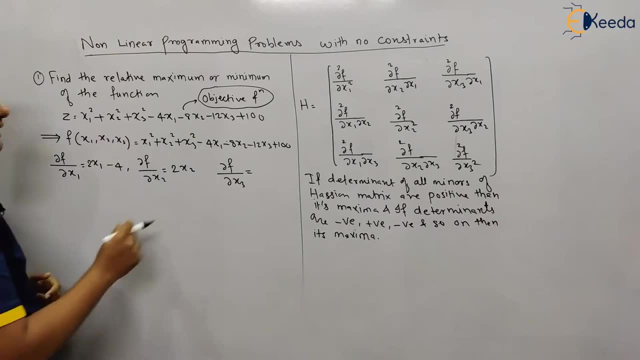 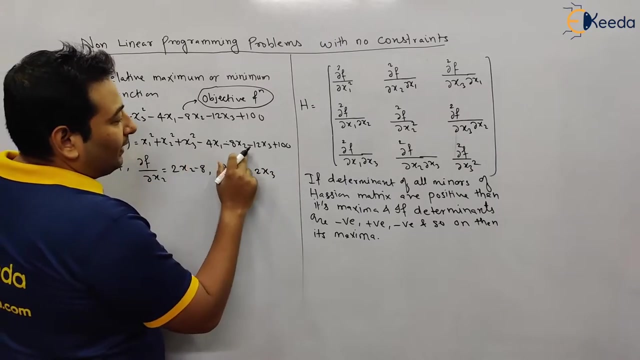 minus 4 will come, and these terms are constant. its derivative is 0. next, dou f upon dou x2, it will be 2x2 and minus 8. and finally, dou f upon dou x3, it will be 2x3, and then we have minus 12. what next? 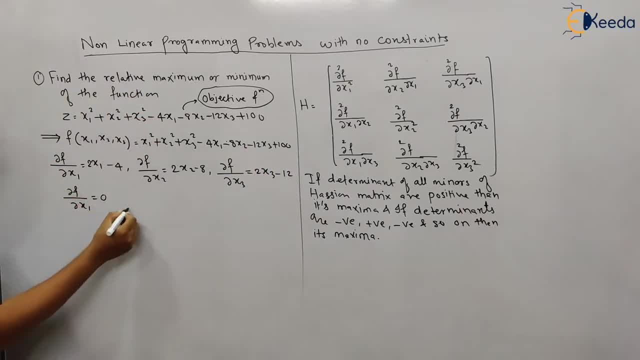 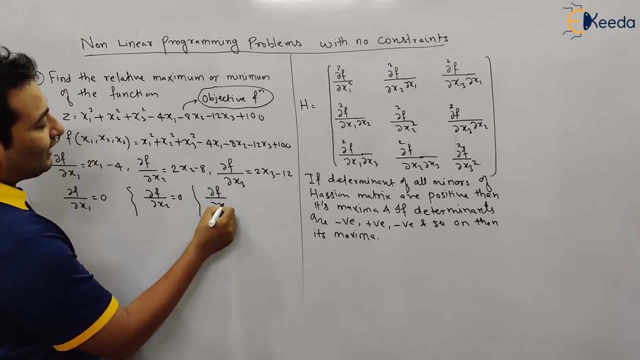 i am going to equate dou f upon dou x1, equal to 0, dou f upon dou x2, equal to 0, and dou f upon dou x3, equal to 0. let us equate. if you equate, this will be 2x1 minus 4, equal to 0. 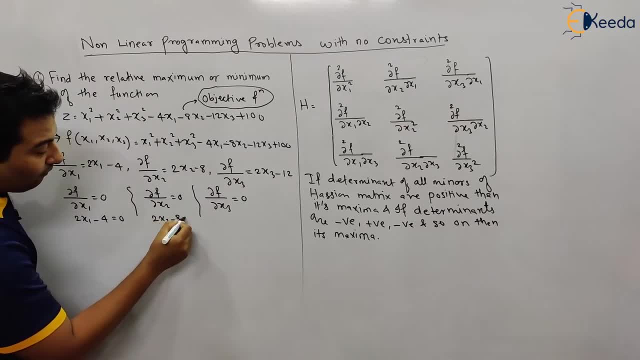 see, remember the procedure if you're going to equate this to 0. and finally, 2 X 3 minus 12 equal to 0. so, from this, X 1 equal to 2, X 2 is equal to 4 and X 3 is. 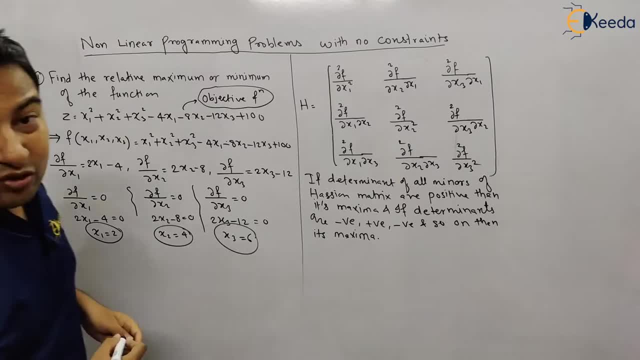 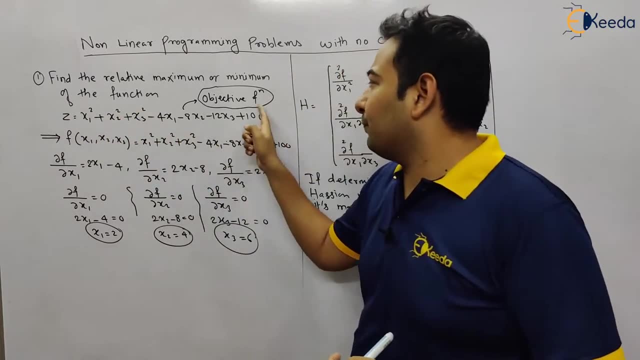 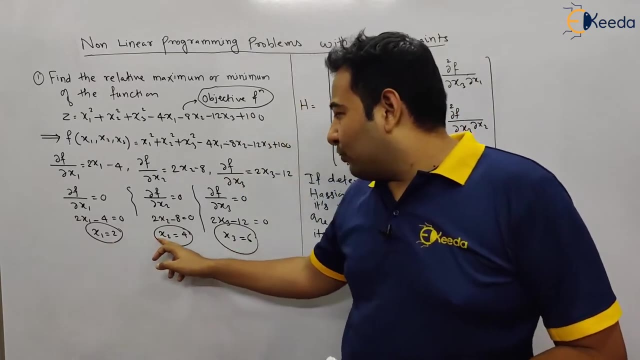 equal to 6. we got the values of X 1, X 2 and X 3. now these values, if I am going to put in the function Z or this function F, I will get a value. if I put X 1, X 2 and X 3 in this particular equation, I'll get the value. 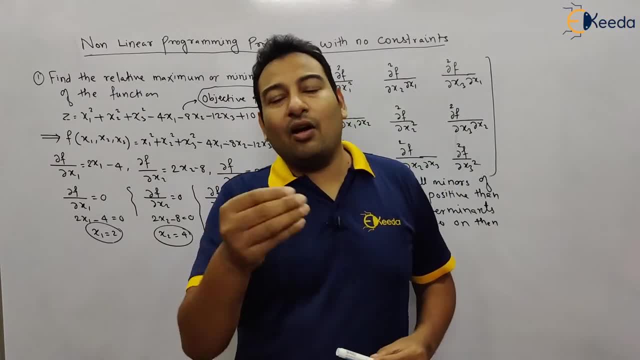 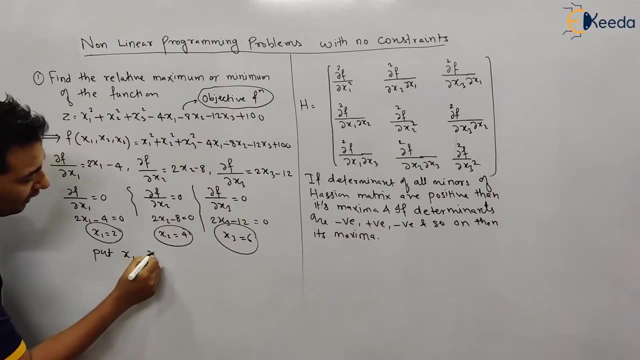 of Z, but that value will be either maxima or minima value. so let us do it. let us do it, put X 1, X 2, X 3 in Z. so if I put X 1, X 2 and X 3 in Z, I am going to. 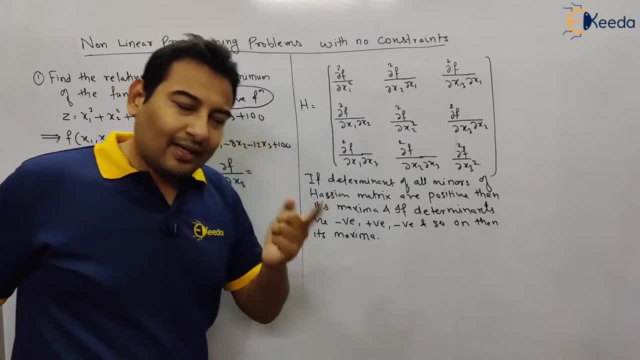 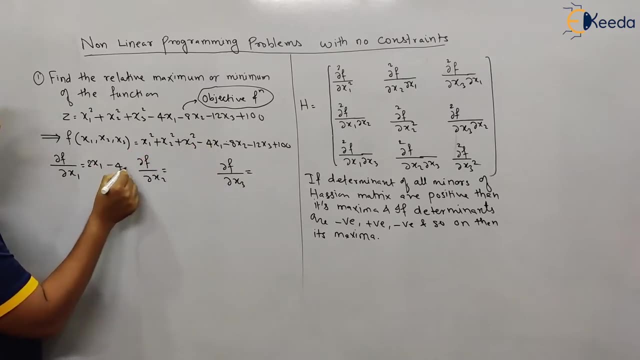 x1, x3- constant. and when you're differentiating with respect to x3, x1, x2 constant. this is 2x1, this is constant, 0, 0 minus 4 because with respect to x1 minus 4 will come and these terms are: 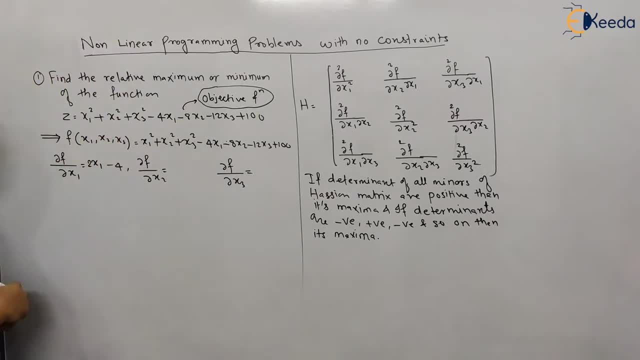 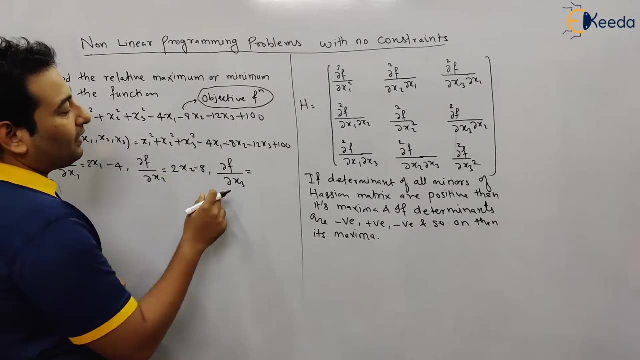 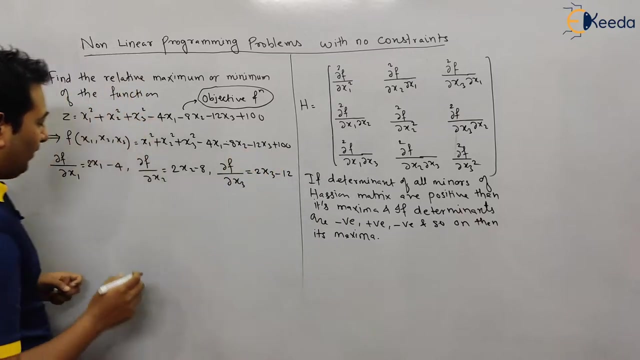 constant. its derivative is 0. next, dou F upon dou x2: it will be 2x2 and minus 8. and finally, dou F upon dou x3: it will be 2x3, and then we have minus 12. what next? I'm going to equate dou F upon dou x1, equal to 0, dou F upon dou x2, equal to 0. 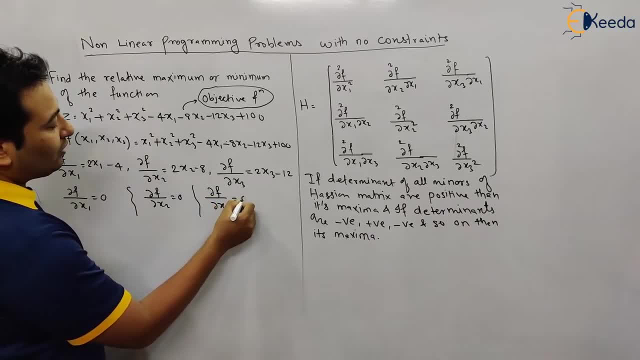 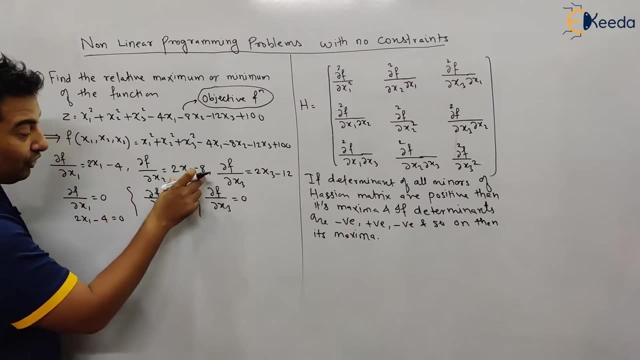 and dou F upon dou x3 equal to 0. let us equate. if you equate, this will be 2x1 minus 4 equal to 0. see remember the procedure if you're going to equate this to 0. and finally, 2x3 minus 12 equal. 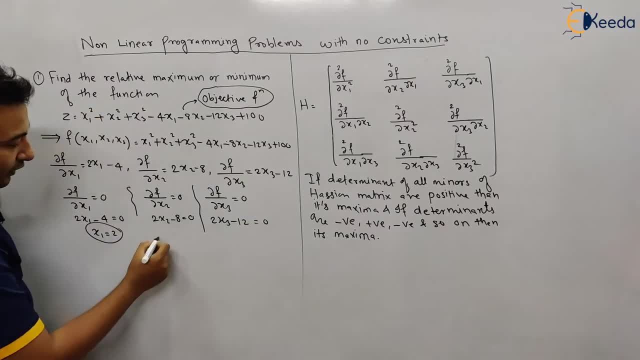 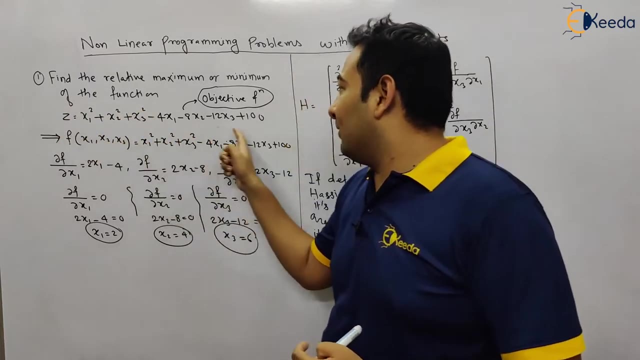 to 0. so from this, x1 equal to 2, x2 is equal to 4 and x3 is equal to 6. we got the values of x1, x2 and x3. now these values, if I'm going to put in the function Z or this function F, I will get a value. 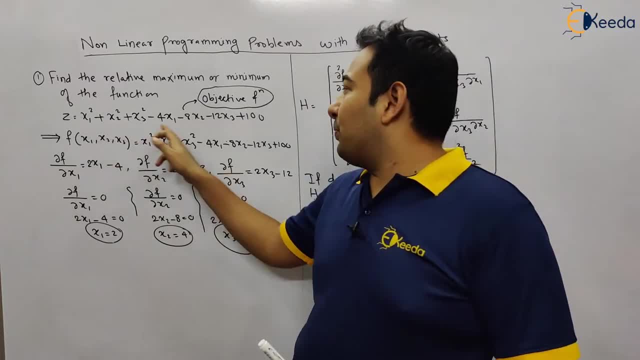 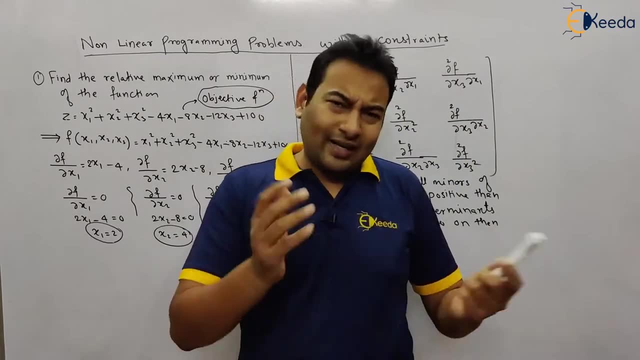 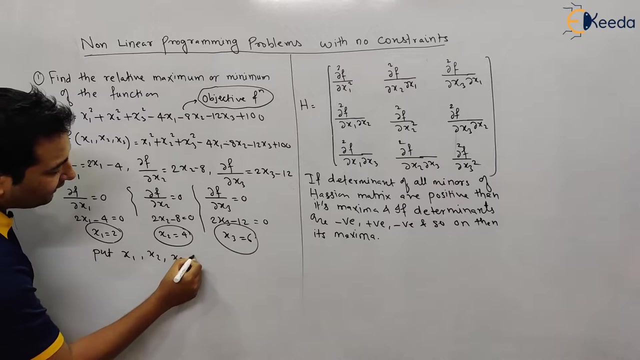 if I'll put x1, x2 and x3 in this particular equation, I'll get the value of Z, but that value will be either maxima or minima value. so let us do it. let us do it. put x1, x2, x3 in Z. so if I put 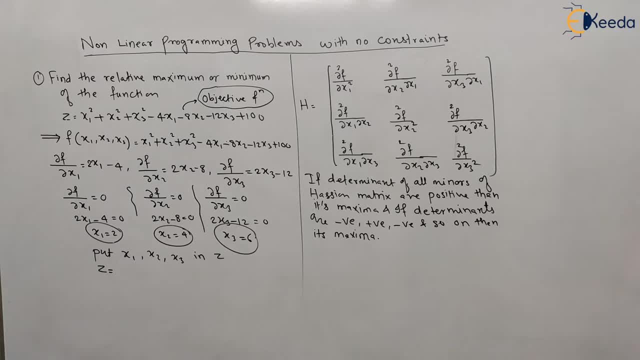 x1, x2 and x3 in Z. I'm going to get a result and that value is 44. you can try by yourself: put and check. you will get the value of Z as 44. how this 2, 4 and 6: put here 2, 4, 6, 2, 4, 6 and so on and try. 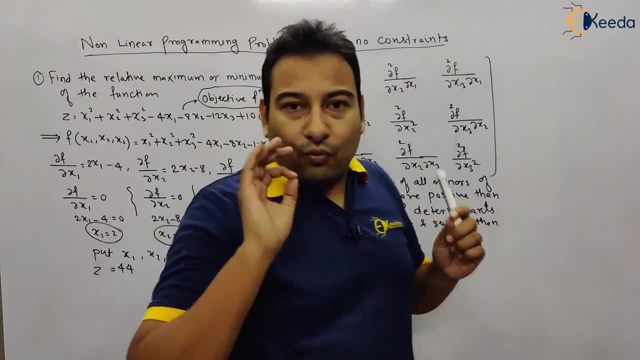 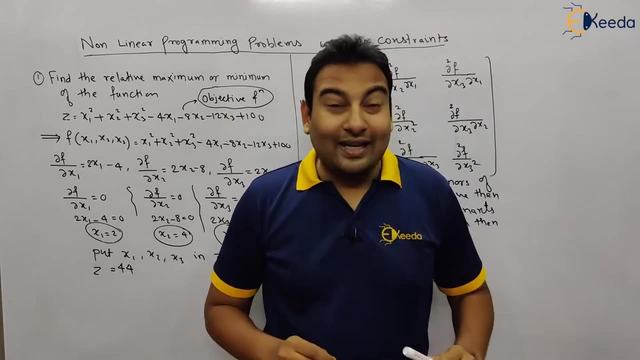 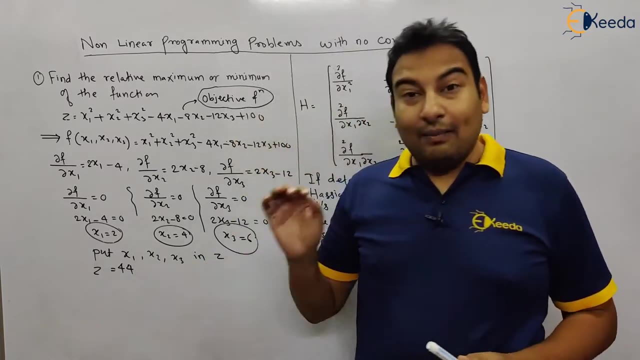 calculating it, you will get the value of Z is equal to 44. so our work is done. we got the value of Z 44. last thing left in this particular problem: that the value that we got is a maximum value or a minimum value. we got the value, but we need to check whether it's a maximum value or a minimum value. 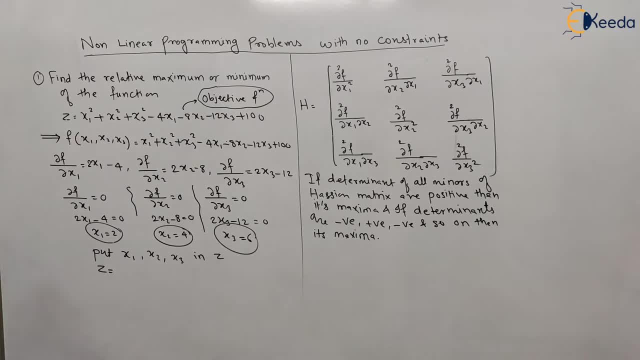 get a result and that value is 44. you can try by yourself. put and check. okay, you will get the value of Z as 44. how this? 2, 4 and 6 put here: 2, 4, 6, 2 4, 6 and. 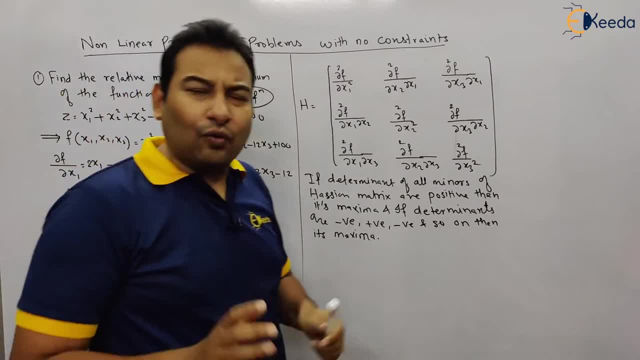 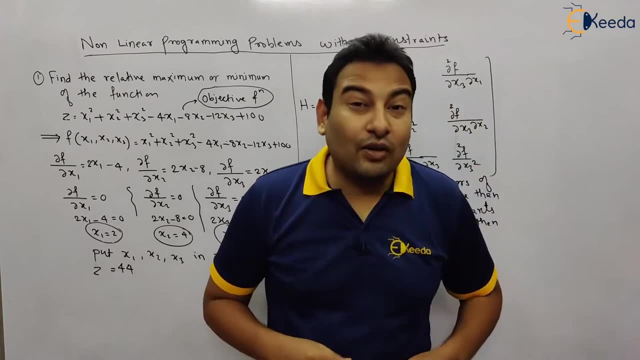 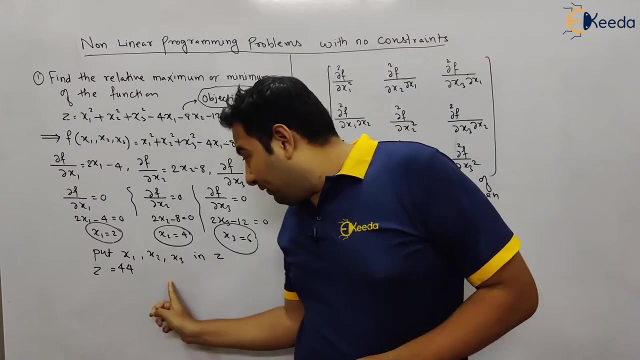 so on and try calculating it, you will get the value of Z is equal to 44. so our work is done. we got the value of Z 44. last thing left in this particular problem: that the value that we got is a maximum value or a minimum value we got. 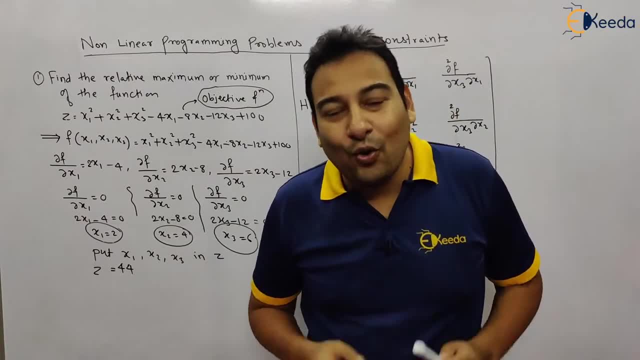 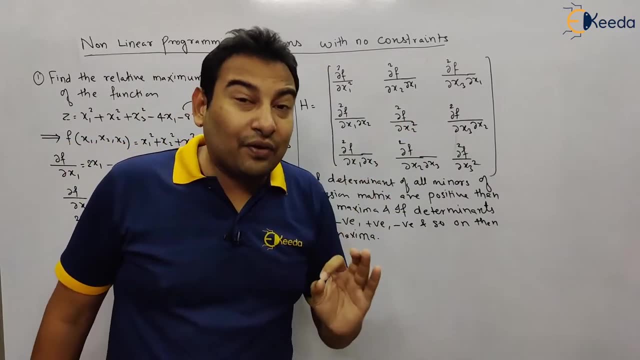 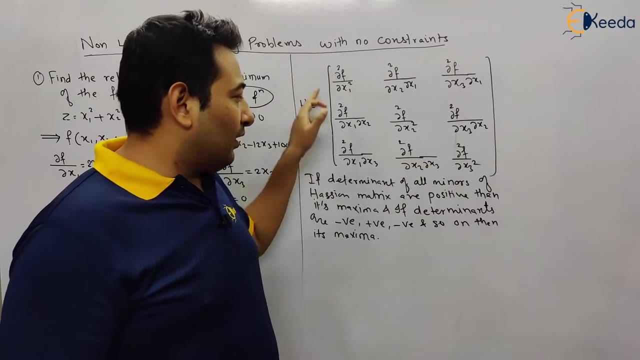 the value, but we need to check whether it's a maximum value or a minimum value. for that purpose, we need to go ahead with the Hessian matrix. Hessian matrix will decide whether the value that we got is a maximum value or its minimum value. for doing that, we need all these values, so let us quickly calculate all. 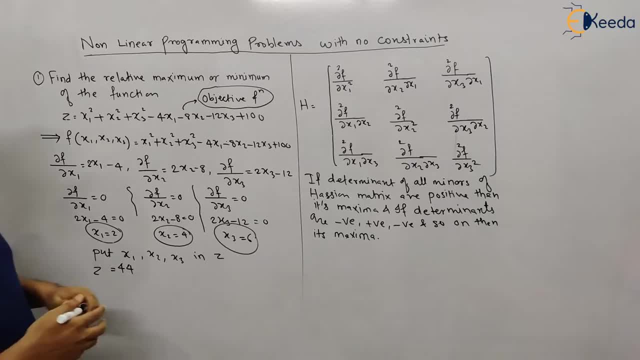 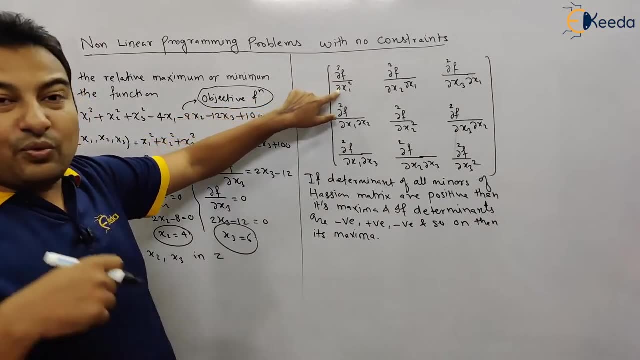 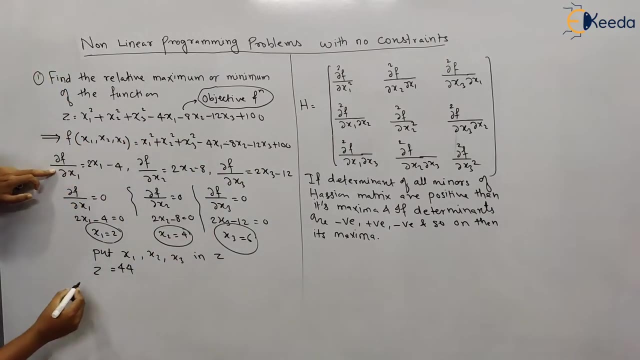 these values. so let's take what we want see here. so this is goes up on 2 x 1 and what we want: those square F upon 2 x1 square. that means we got o F upon x1. we need to differentiate one more time with respect to x1 to get dou square f upon 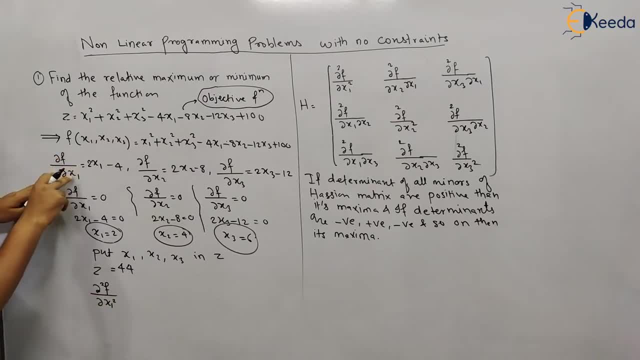 dou x1 square. dou f upon dou x1 will be differentiated once again with respect to x1, so that is 2.. if i am going to differentiate with respect to x1, this is 2 and minus 4 derivative is 0. what else next term i want see here? i want dou square f upon dou x2 square. that means this term. 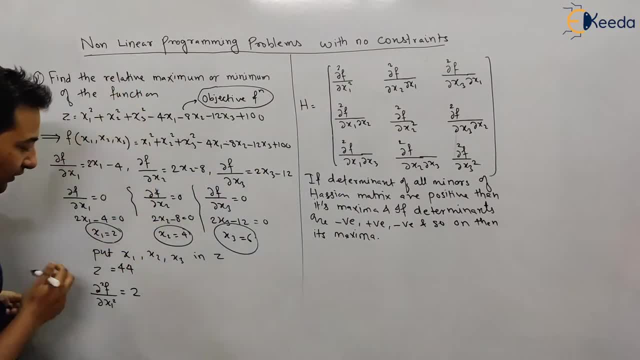 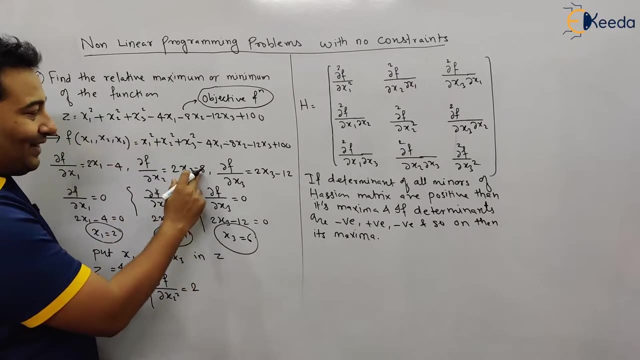 i am going to again differentiate with respect to x2. therefore it will be dou square f upon dou x2 square equal to: if we differentiate this, this term, with respect to x2, here it is 2: x2 derivative is 1 and minus that derivative is 0. what else? 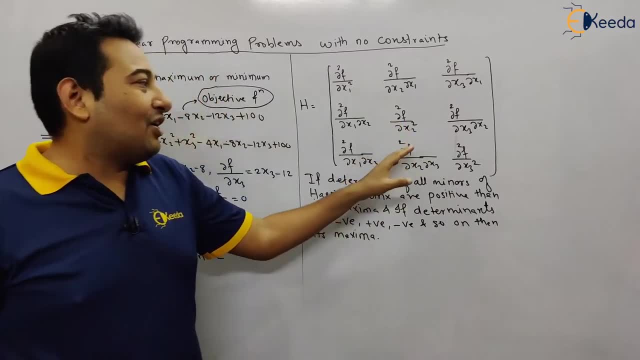 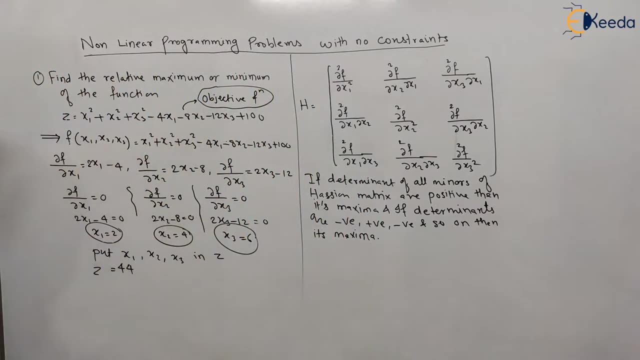 for that purpose, we need to go ahead with the Hessian matrix. Hessian matrix will decide whether the value that we got is a maximum value or it's a minimum value. for doing that, we need all these values. so let us quickly calculate all these values. so let's take what we want see here. so 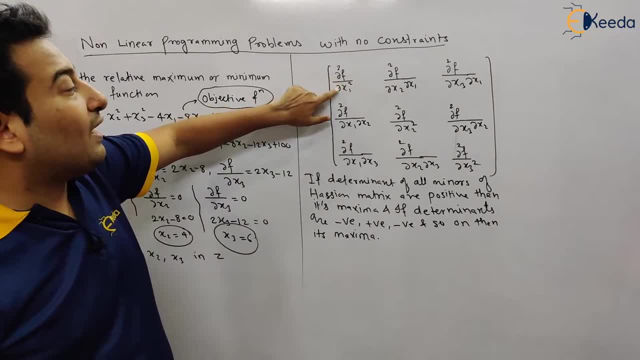 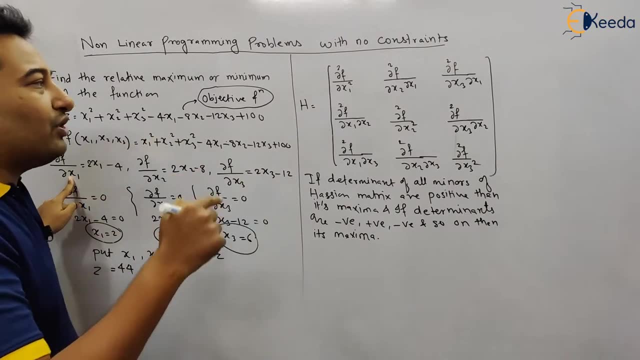 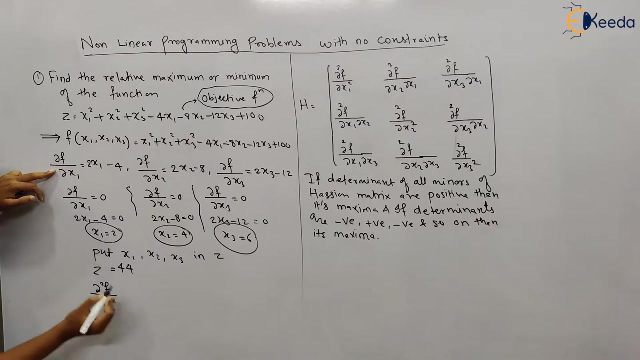 this is dou f upon dou x1 and what we want: dou square f upon dou x1 square. that means we got dou. we need to differentiate one more time with respect to x1 to get dou square f upon dou x1 square. dou f upon dou x1 will be differentiated once again with respect to x1, so that is 2. 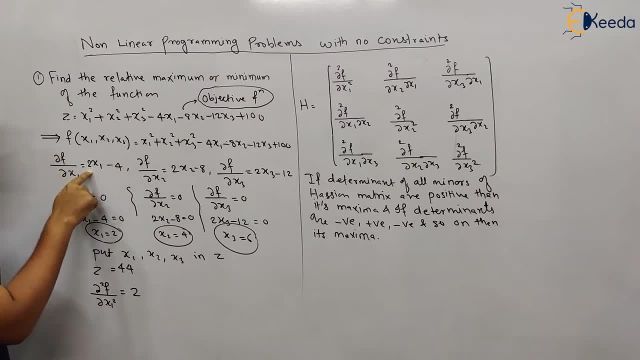 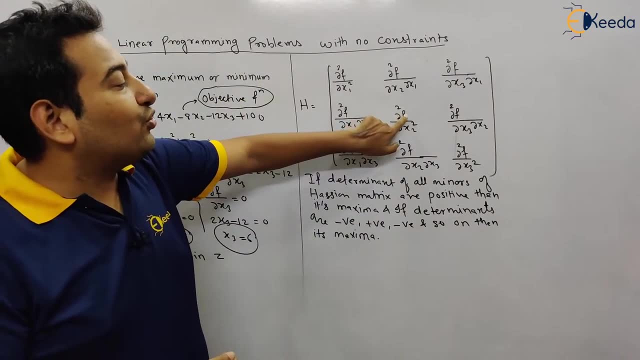 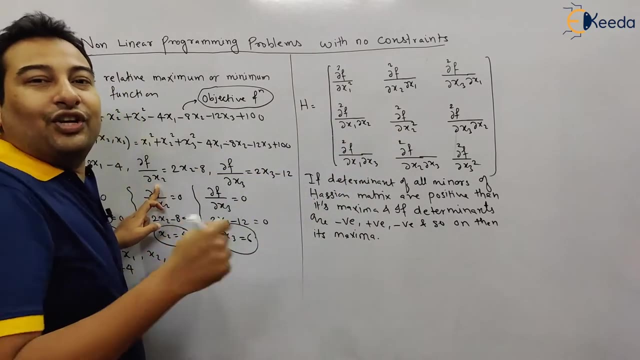 if I'm going to differentiate with respect to x1, this is 2 and minus 4 derivative is 0. what else next time? I want c here I want dou square, f upon dou x2 square. that means this term. I am going to again differentiate with respect to x2. 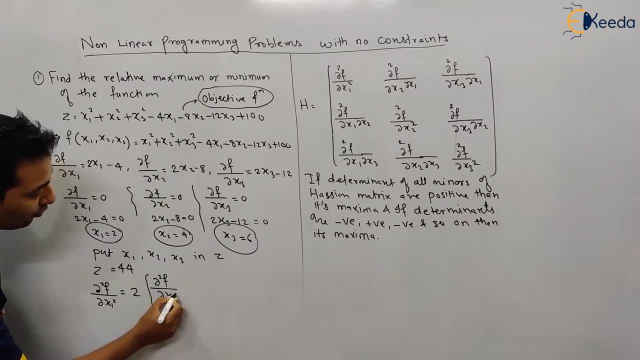 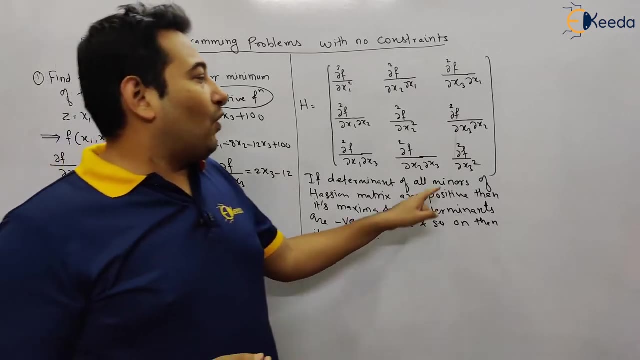 therefore, it will be dou square f upon dou x2 square, equal to: if we differentiate the this term with respect to x2, here it is 2 x2 derivative is 1 and minus a derivative is 0. what else? let us check. we want this particular term: dou square f upon dou x3 square. 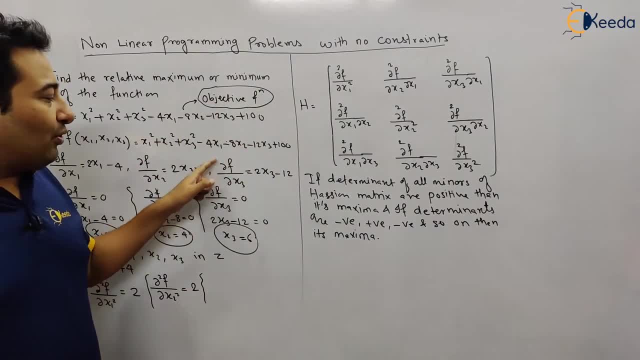 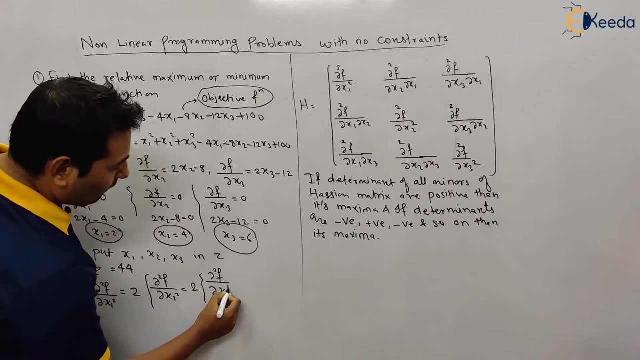 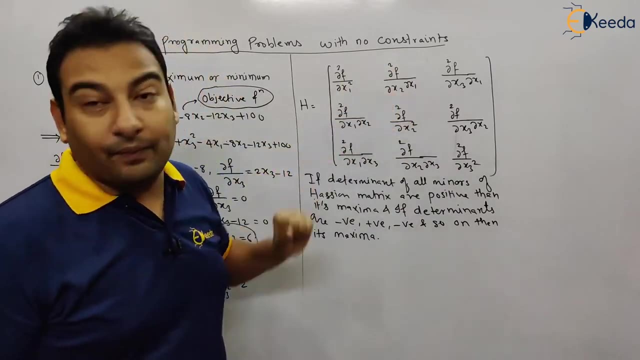 What needs to be done? See dou f upon dou x3,. we already have one more derivative with respect to x3.. So that will be again 2.. What else See? we got these terms. Let us find it out, this particular term. 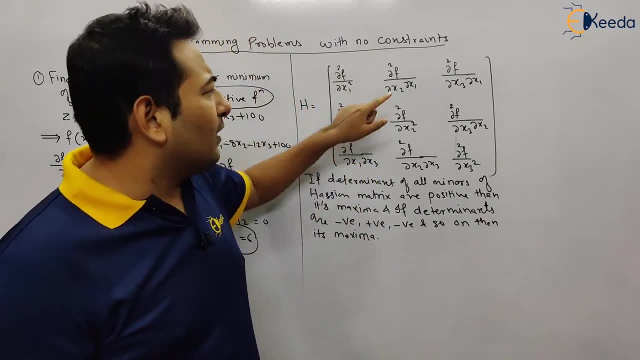 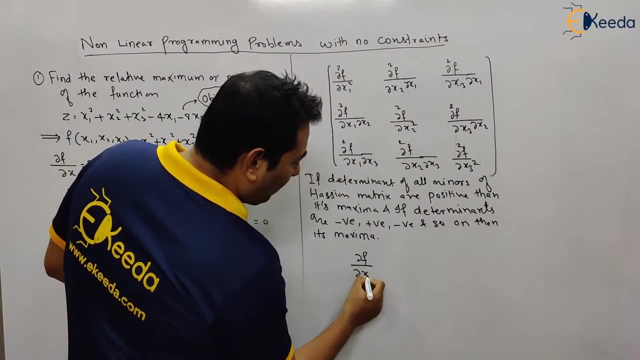 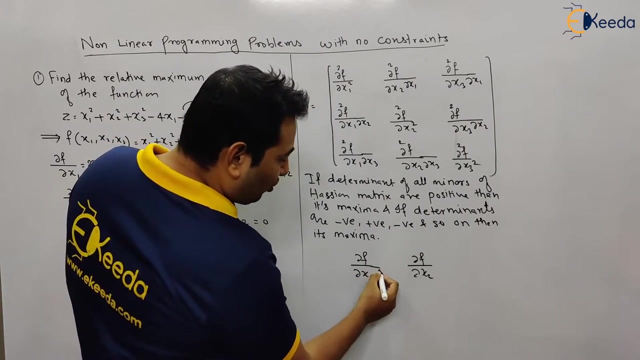 What does this term indicate? See here, it's very simple. It means that let me write down here: See, we already have dou f upon dou x1 and we already have dou f upon dou x2.. This term, if you differentiate with respect to x2, or this term you differentiate with respect to x1, doesn't matter. 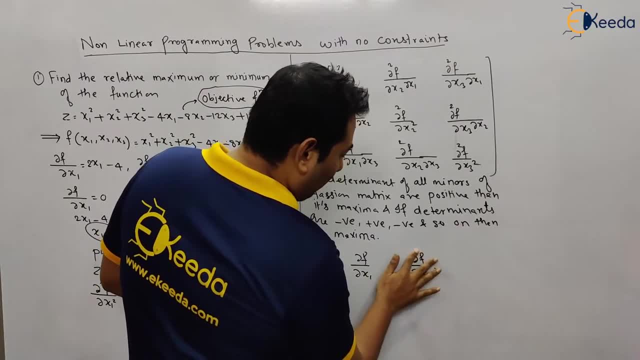 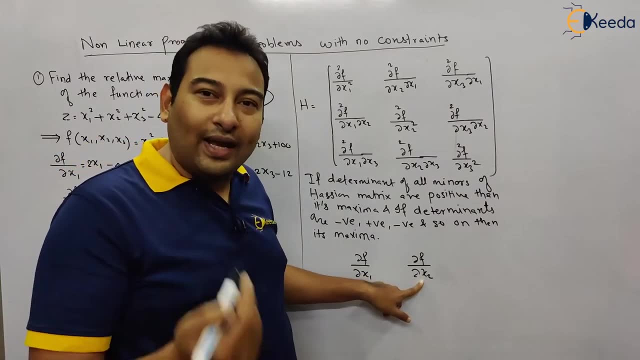 So one and the same thing, What I am saying. See here: either you differentiate this term with respect to x2 or this term with respect to x1.. Ultimately, you will get this value. See, both the values are the same. 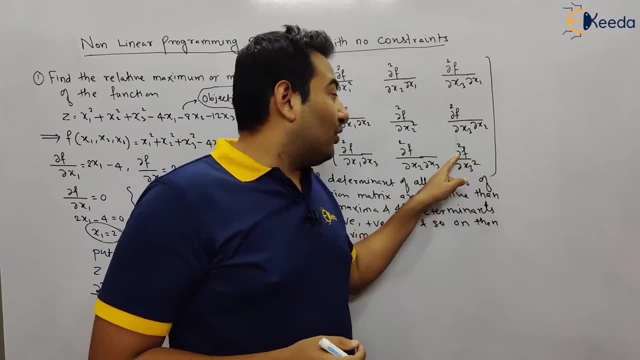 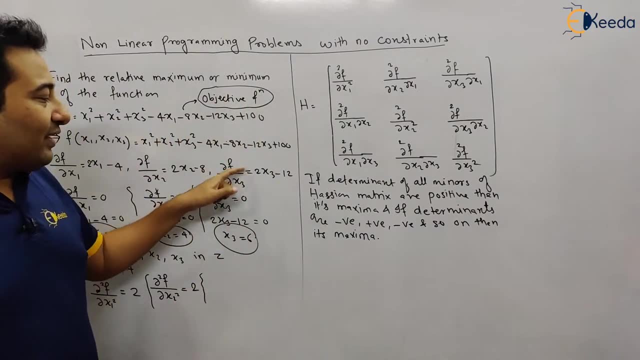 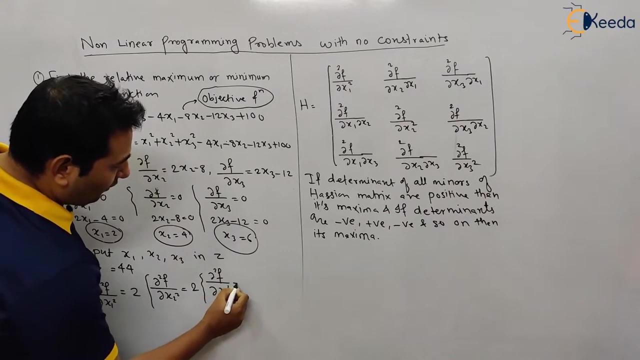 let us check. we want this particular term: dou square f upon dou x3 square. what needs to be done? see dou f upon dou x3. we already have one more derivative with respect to x3, so that will be again 2. what else? see, we got these terms. let us find it out, this particular term. 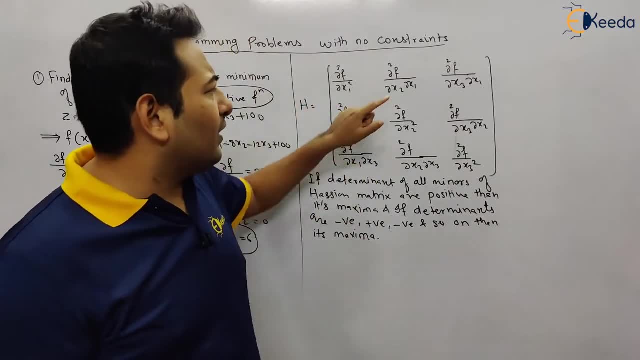 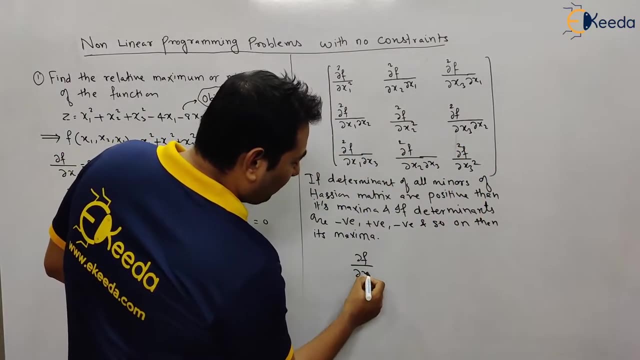 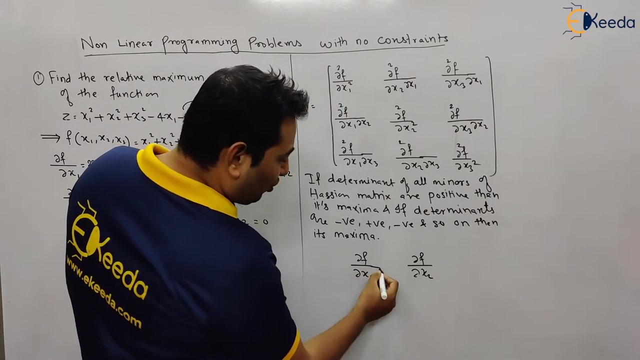 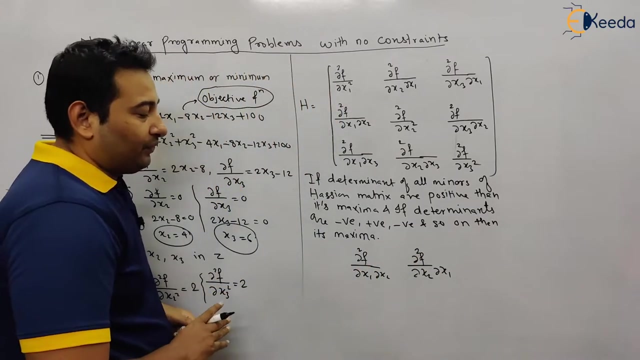 what does this term indicate? see here, it's very simple. it means that let me write down here: see, we already have dou f upon dou x1 and we already have dou f upon dou x2, this term. if you differentiate with respect to x2 or this term, you differentiate with respect to x1 doesn't matter, so one in the same. 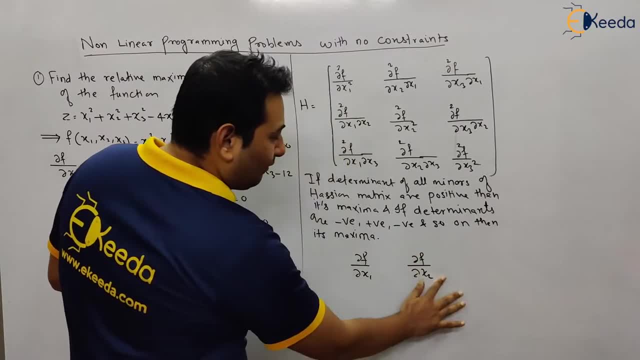 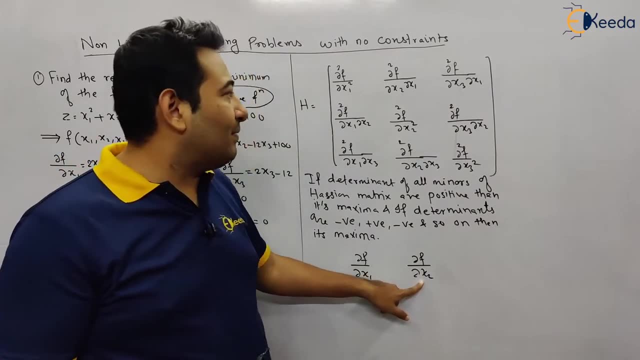 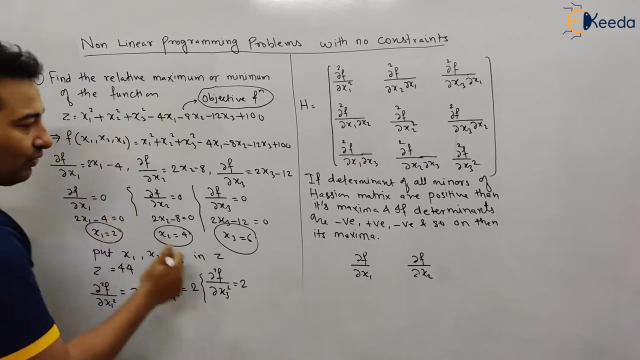 what i'm saying. see here: either you differentiate this term with respect to x2 or or this term with respect to x1. ultimately you will get this value. see, both the values are same. let us do it for both the terms. see here: it is 2x1 minus 4. 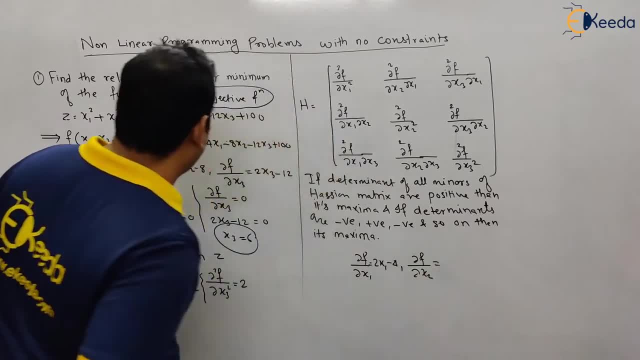 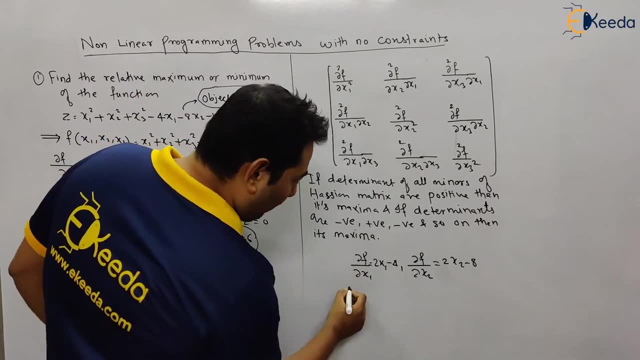 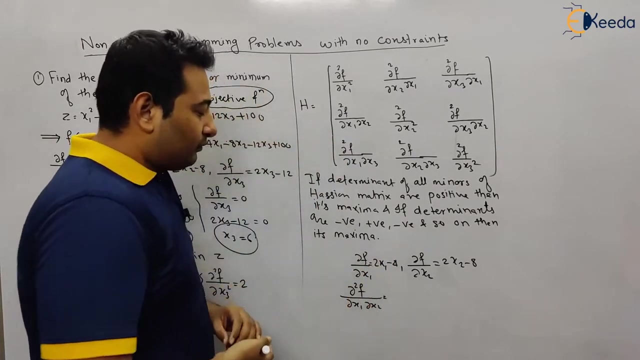 so there should be no confusion. dou f upon dou x2 is a 2x2 minus 8. see here whether you differentiate this term with respect to x2. so if you differentiate with respect to x2 with respect to x2, if you differentiate, that means x1 is a constant. its derivative will: 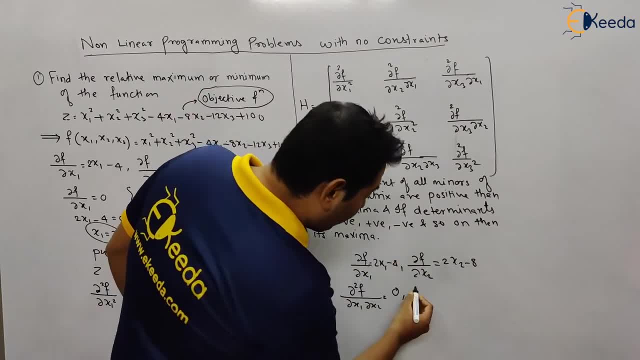 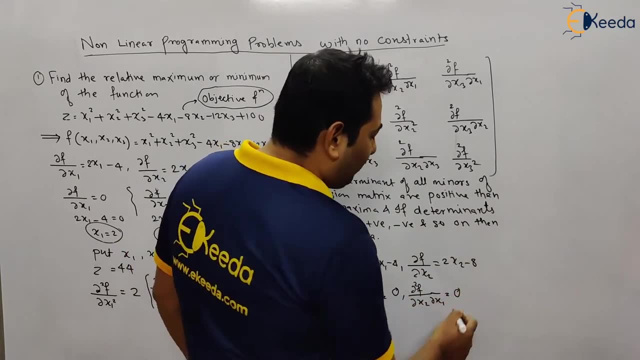 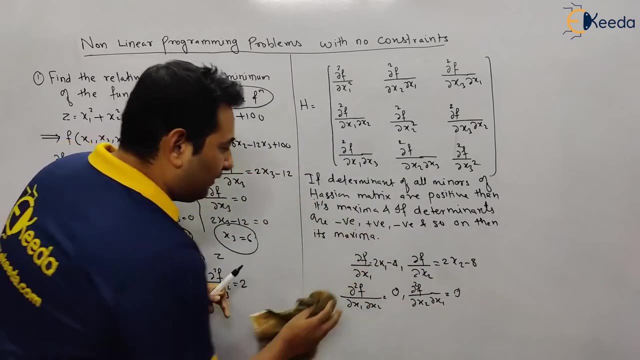 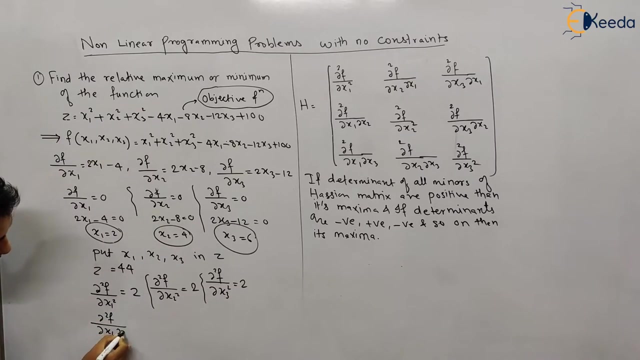 be 0, or this is your term. you can differentiate with respect to x1. if you differentiate with respect to x1, its derivative is 0. see here: whatever you do, you will get the answer as 0. so let us write it down here: dou square f upon dou x1, dou x2 is equal to 0. i hope this is clear. next, what about? 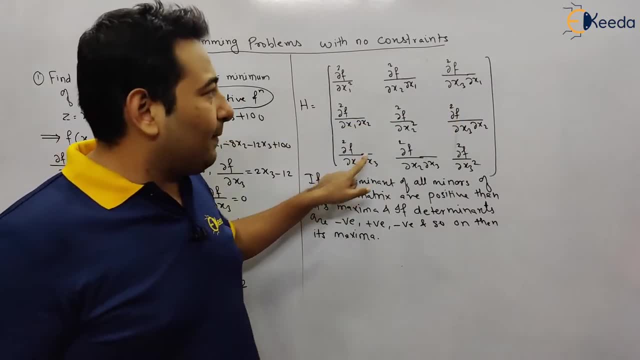 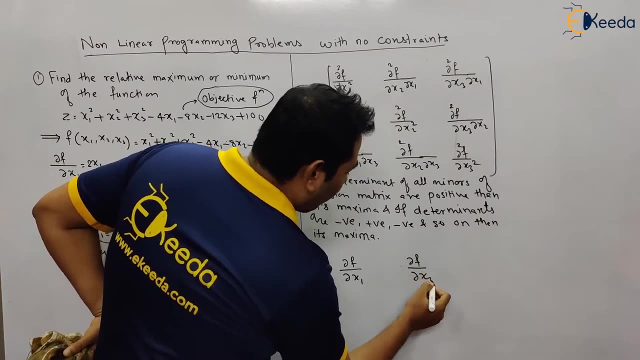 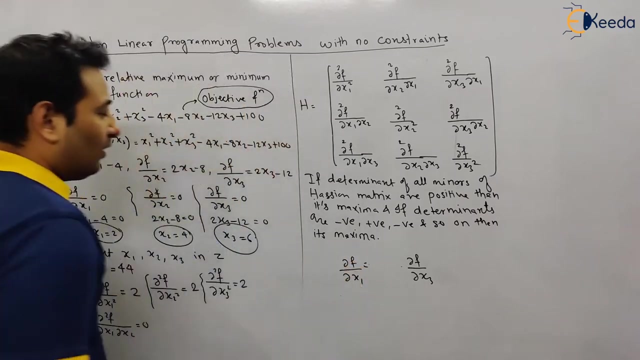 this term, these two terms, simply again the same. see dou f upon dou x1 or dou f upon dou x3. if you differentiate this term with respect to x3 or this term with respect to x1, one in the same thing, see here. what is that i am? 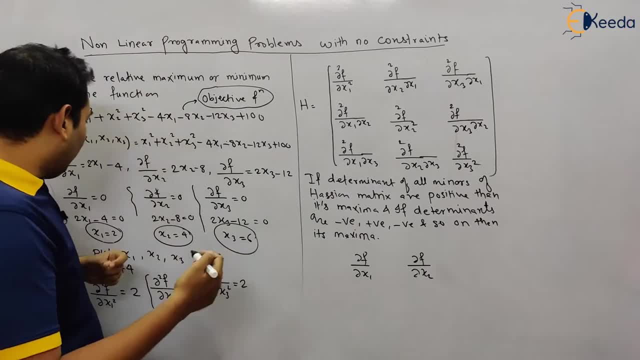 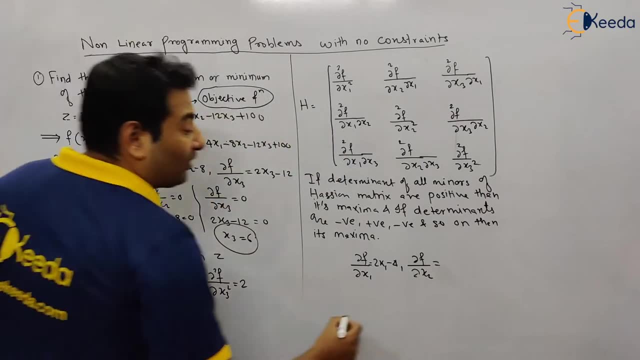 Let us do it for both the terms. See here: it is 2x1 minus 4.. So there should be no confusion. Dou f upon dou x2 is 2x2 minus 8.. See here whether you differentiate this term with respect to x2.. 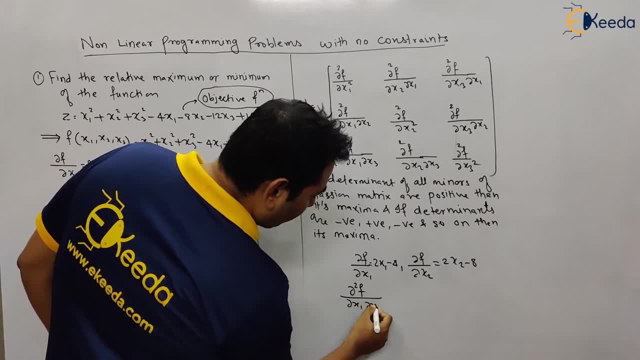 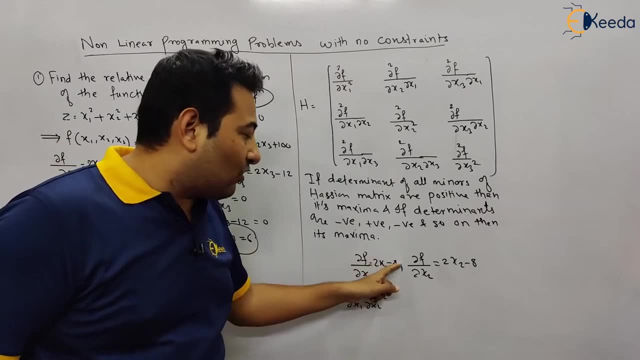 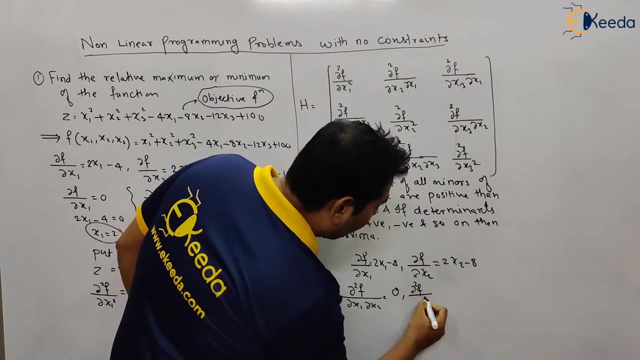 So if you differentiate with respect to x2, that means x1 is a constant- its derivative will be 0.. Or this is your term- You can differentiate with respect to x1.. If you differentiate with respect to x1, its derivative is 0.. 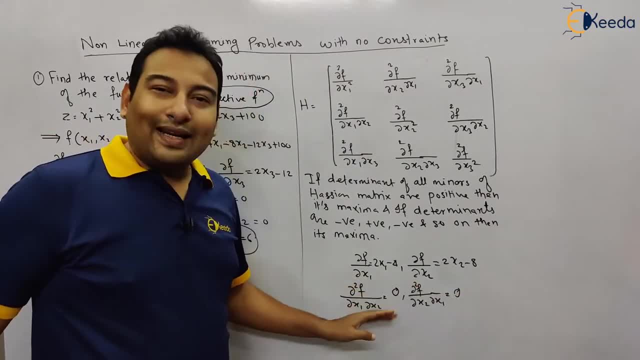 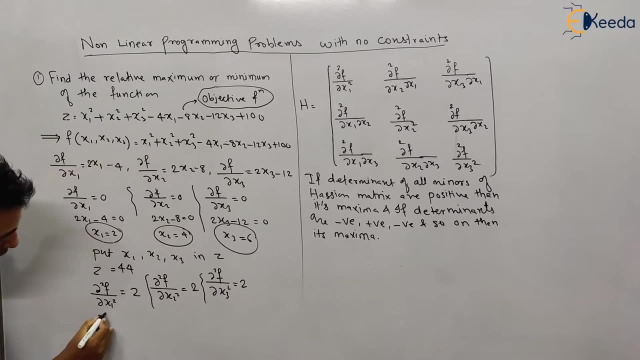 See here, whatever you do, you will get the answer as 0.. So let us write it down here: Dou square f upon dou x1, dou x2 is equal to 0.. I hope this is clear. Next, What about this term? 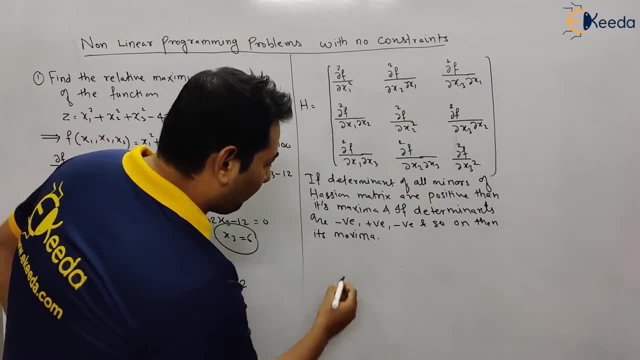 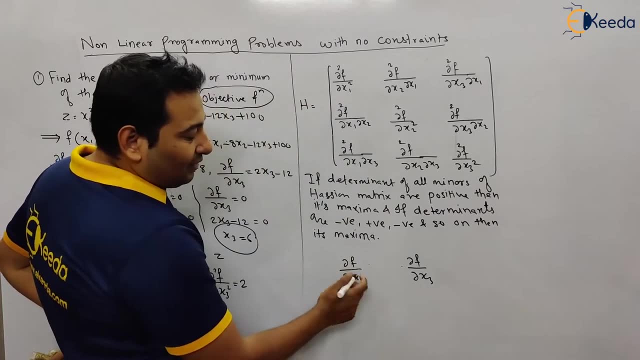 These two terms Simply again the same. See dou f upon dou x1 or dou f upon dou x3.. If you differentiate this term with respect to x3 or this term with respect to x1, one and the same thing. 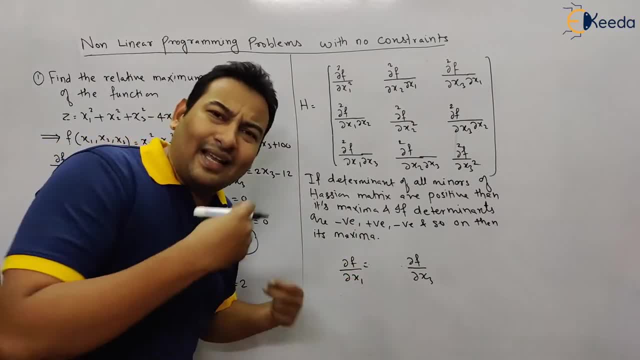 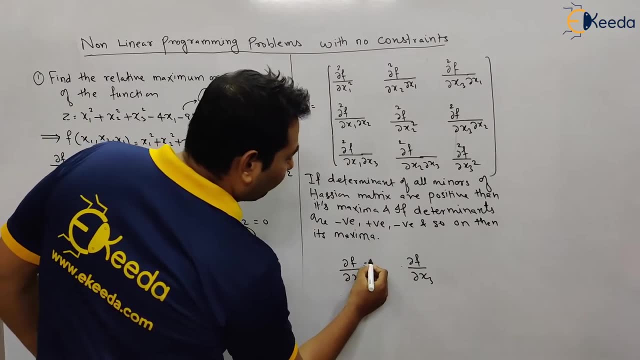 See here: What is that? I am explaining this in detail. In the next problems onwards we will be doing it directly: Dou f upon dou x1, the value is 2x1 minus 4.. See here: Dou f upon dou x3, the value is 2x3 minus 12.. 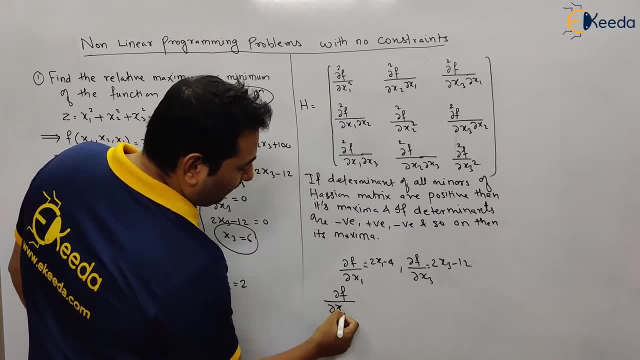 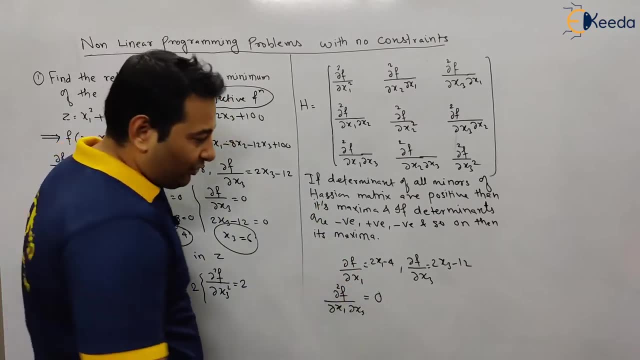 Now you differentiate this with respect to x3.. See here, With respect to x3, if you differentiate, x3 is variable, rest, everything is a constant Derivative is 0.. Or this x3 with the x1, again it is 0.. 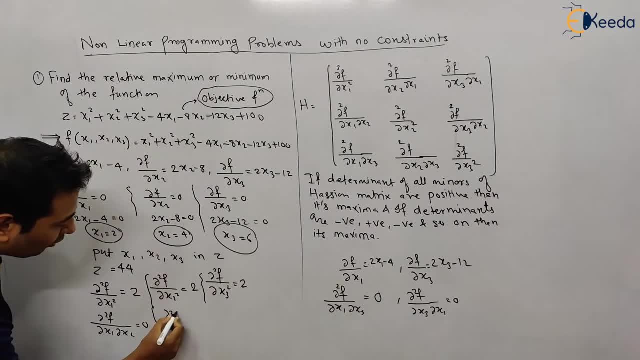 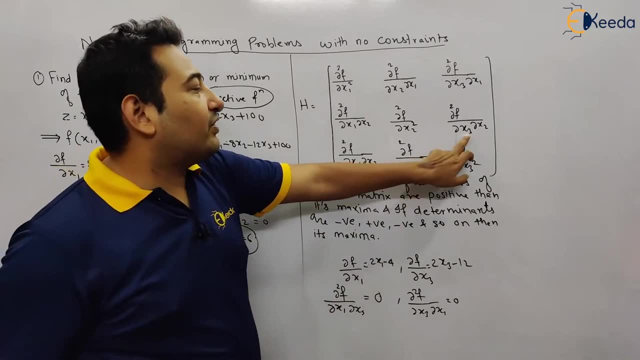 So, whatever you do, the answer will be 0.. So here, dou square f upon dou x1, dou x3 will be equal to 0.. And the same way, Finally, x3 and x2, or, this term, x2 or x3. 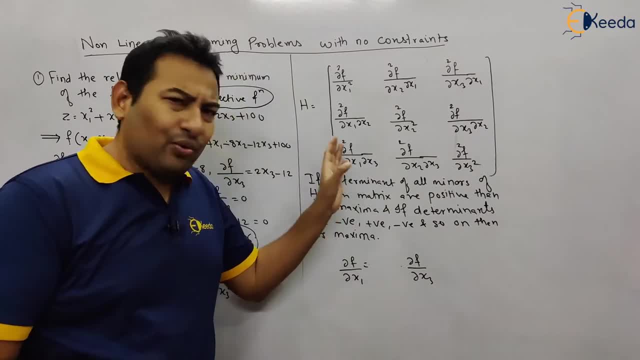 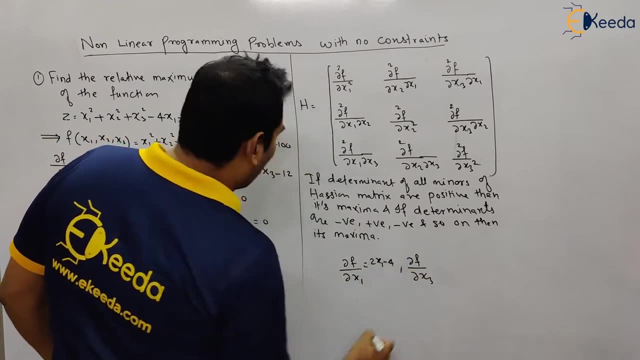 explaining here in this in detail. in the next problems onwards will be doing it directly: dou f upon dou x1, the value is 2x1 minus 4. see here. dou f upon dou x3, the value is 2x3 minus 12. now you differentiate. 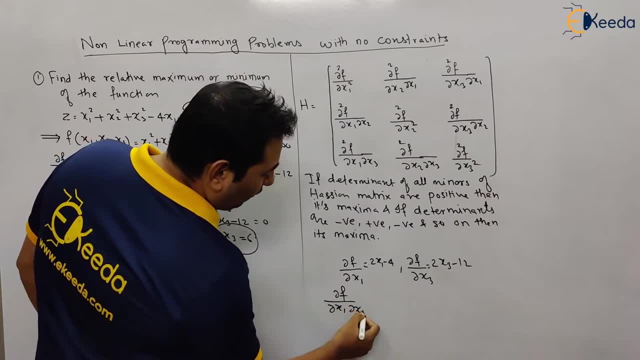 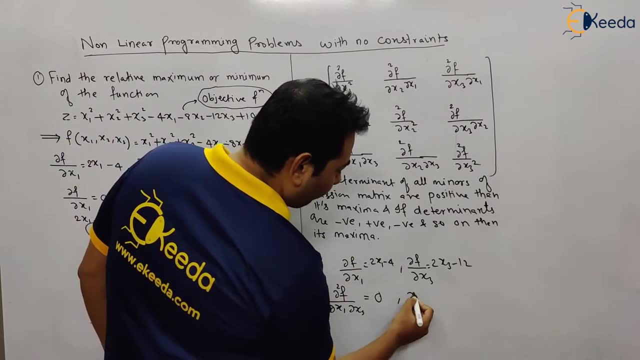 this with respect to x3. see here with respect to x3. if you differentiate, x3 is variable, rest, everything is a constant derivative is zero. or this x3 with x1 later is 0, the Falcon derivative are 0. or When x1 is 0, the absolute value of. twice is equal to one and this y0 is just 1, so this is what you shouldり. I am spec first his already6 x2 equals換 0. nothing is号자맛 ivדαu the whole. What does he mean? by what is this? 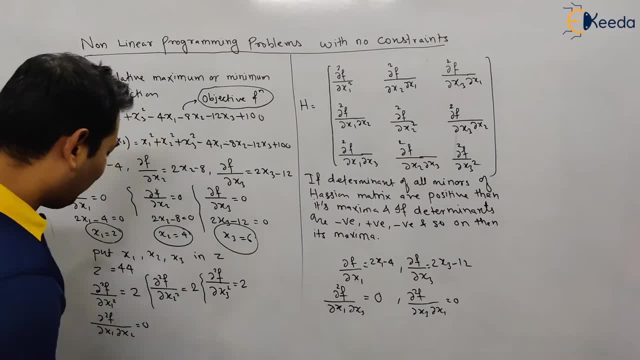 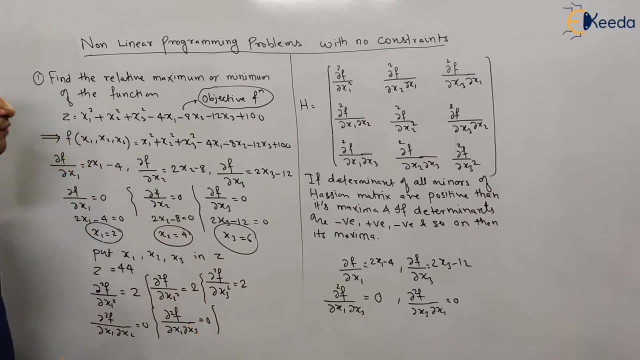 x1, again it's 0. so whatever you do, the answer will be 0. so here dou square f upon dou x1, dou x3 will be equal to 0 and the same way. finally, x3 and x2, or, this term, x2 or x3, see here. 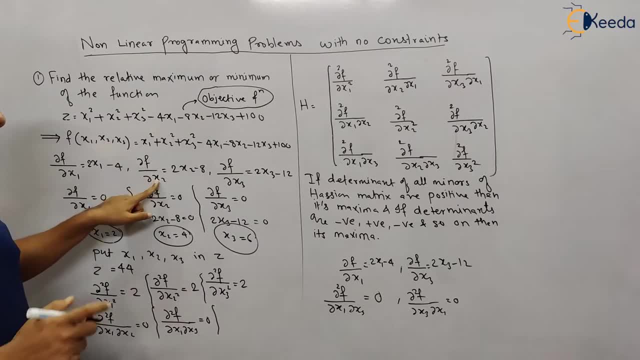 this is x2, you can differentiate with respect to x3. or this is x3, you can differentiate with respect to x2. ultimately, you're going to get the same thing. so this is the term if i'm going to differentiate with respect to x3. this is constant. its derivative will be 0. so, in short, 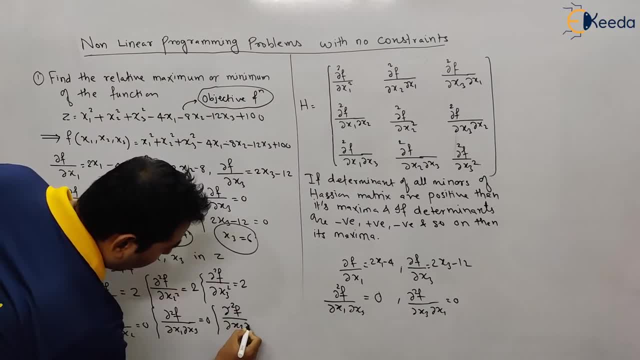 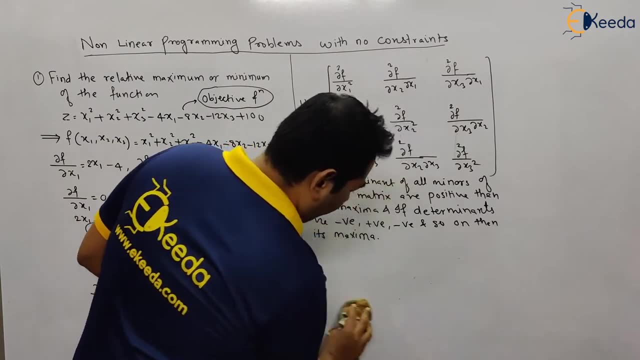 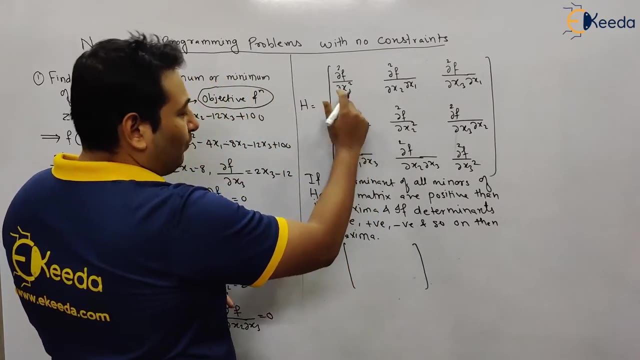 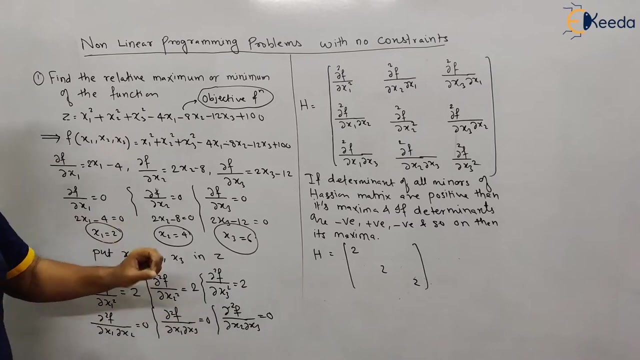 dou x2, dou x3, its derivative will be equal to 0. so let us put all the values that we got. so h equal to this value. we got it as 2, 2 and 2, see here. so rest every value, rest all the values, see all these values are 0, see here. we have already calculated. 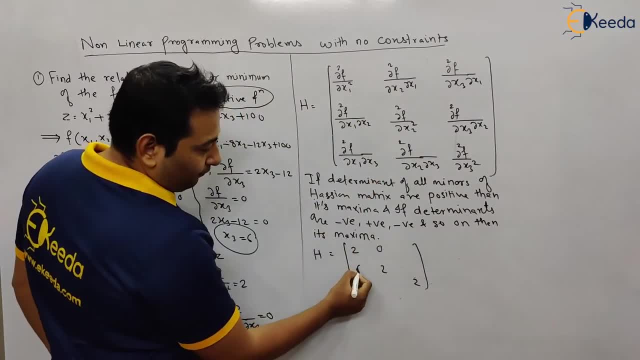 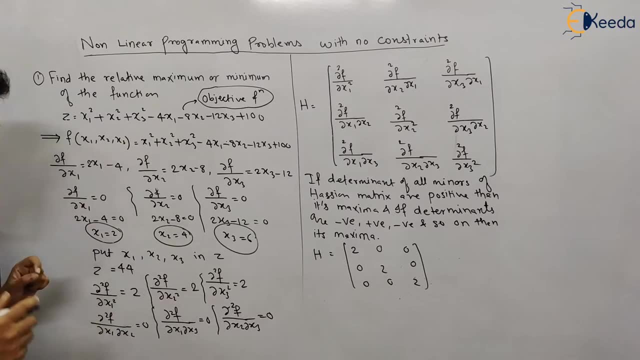 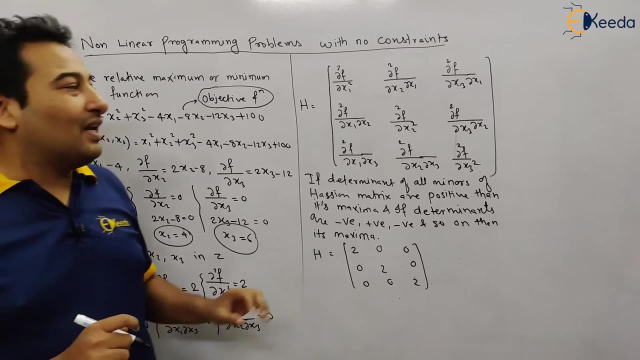 because this term is same as this, this is same as this and this is same as this. so this is h. see, friends, we already got the solution. i just need to check what to write here: maxima or minima. for that purpose, we are going to use hessian matrix, okay, so see the definition that i have. 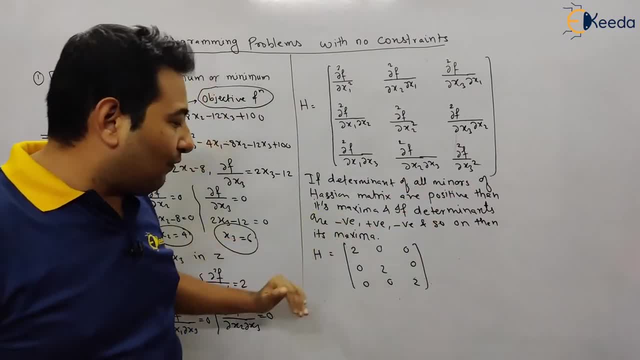 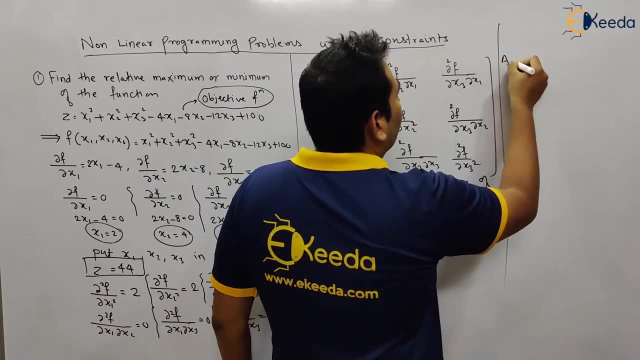 written here. if determined by the definition of hessian matrix, we are going to use hessian matrix, so hessian matrix in kth and over nth cannot be derived from something. if t is general, say hm of time minus one twenty twelve integral. take mod fl blo, the partial元 per first. 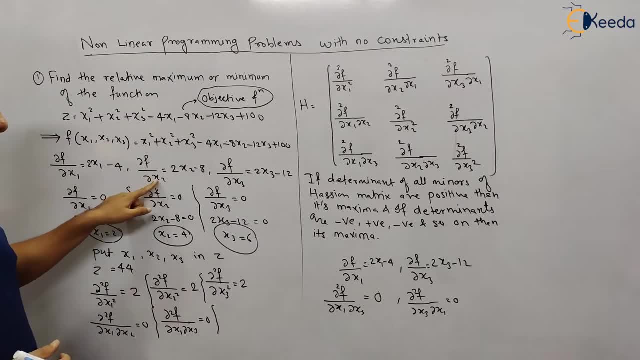 See here: This is x2.. You can differentiate with respect to x3, or this is x3.. You can differentiate with respect to x2.. Ultimately, you are going to get the same thing. So this is the term. If I am going to differentiate with respect to x3, this is constant. 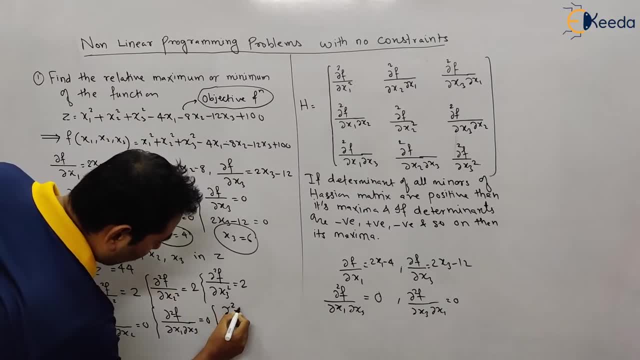 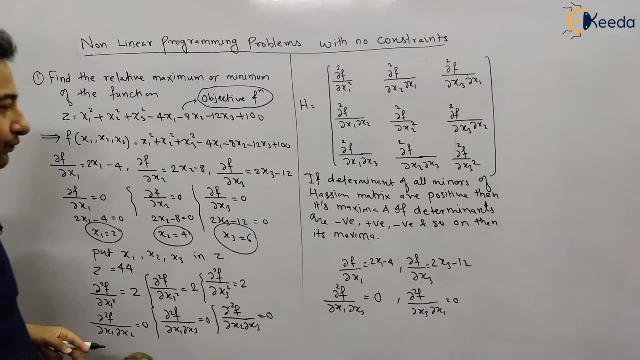 Its derivative will be 0.. So, in short, dou x2, dou x3.. Its derivative will be 0.. Its derivative will be 0.. Its derivative will be 0.. So let us put all the values that we got. 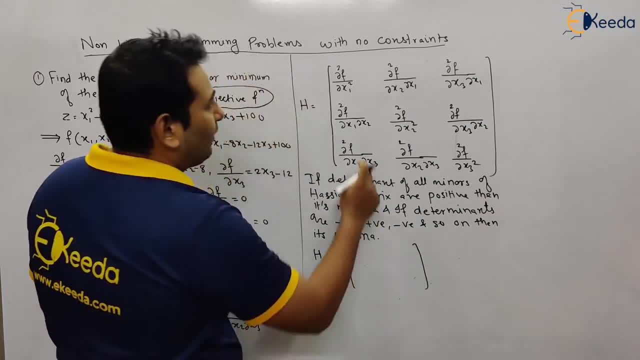 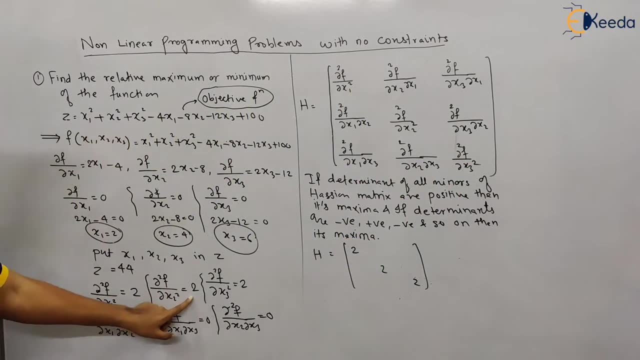 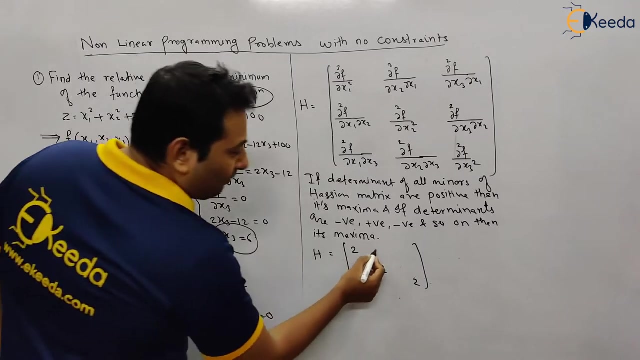 So h equal to this value, We got it as 2.. 2 and 2, see here. Rest every value. Rest all the values. See all these values are 0, see here: We have already calculated because this term is same as this. 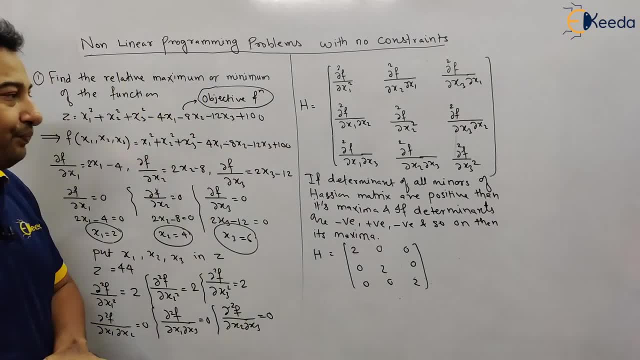 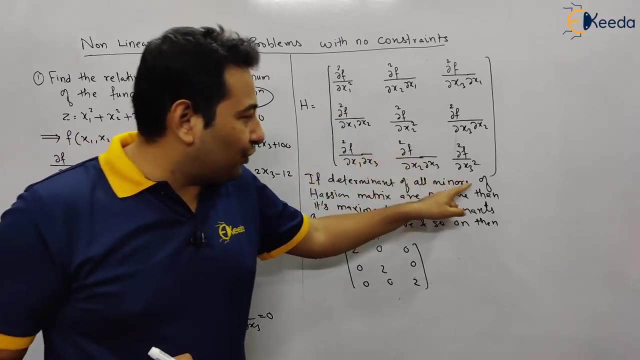 This is same as this. this is same as this. so this is H. see, friends, we already got the solution. I just need to check what to write here: maxima or minima. for that purpose, we are going to use Hessian matrix, okay, so see the definition that I have written here. 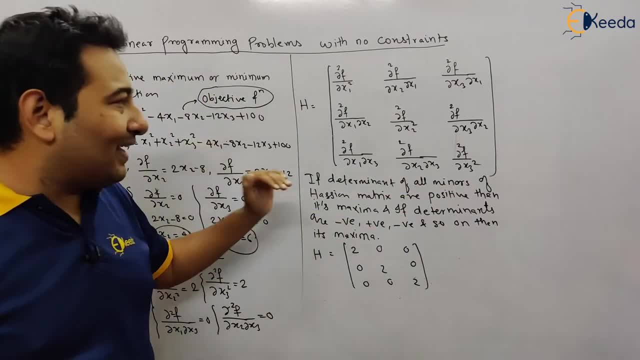 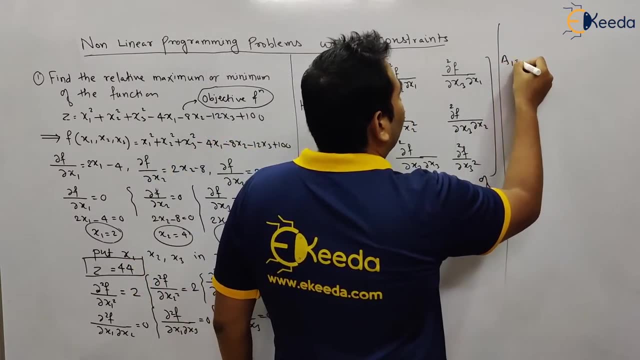 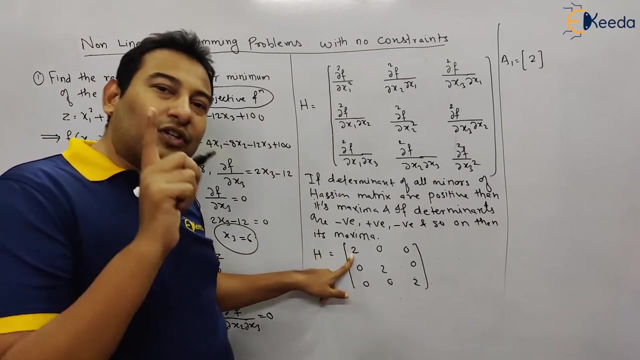 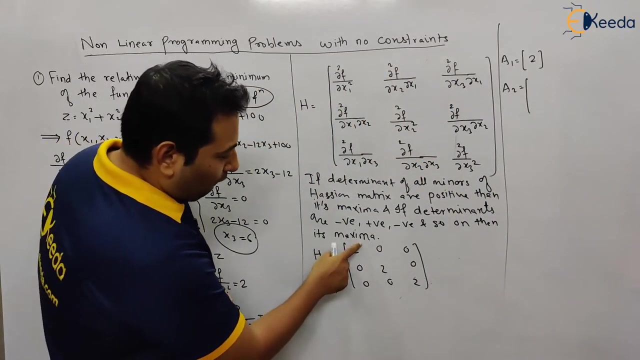 if determinant, of all miners. first of all, there are three miners here. so what are the three miners involved in the problem? the first miner- let's say a one- is this: first row first column is your first miner. second miner means first row, first column. one miner second. 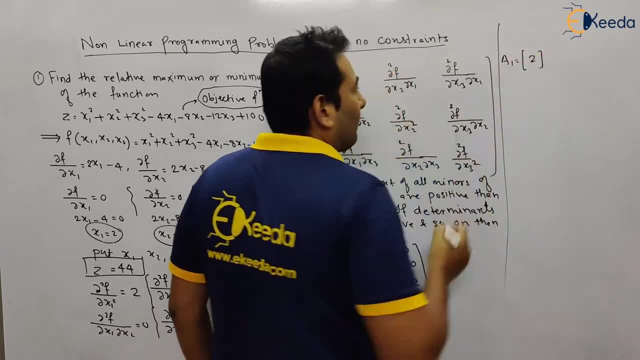 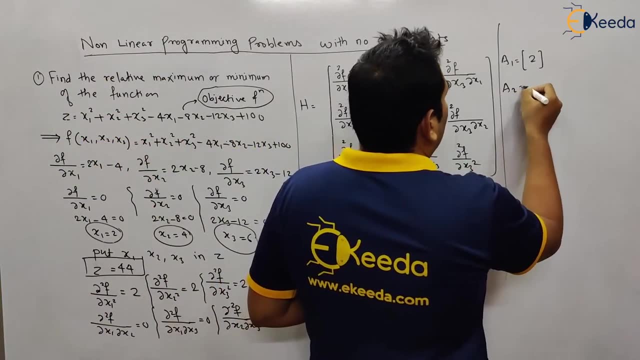 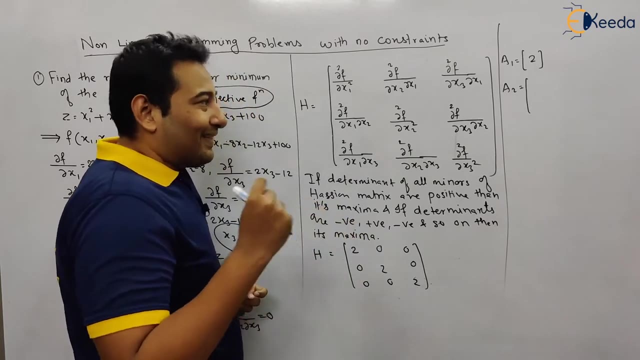 term is theuel minus equal to a minus one, since our final product is 0. and then this you're going to find hessian matrix leagues, bin puta, minusizada variables. minus for twice the termials gives you plus or minus 2, right. so what will this a minus to you give us a minus b, is it from m to d? and what does that represents then? what will that means? r minus 1 tfloff kg lagi other terms which are also involved in this від. 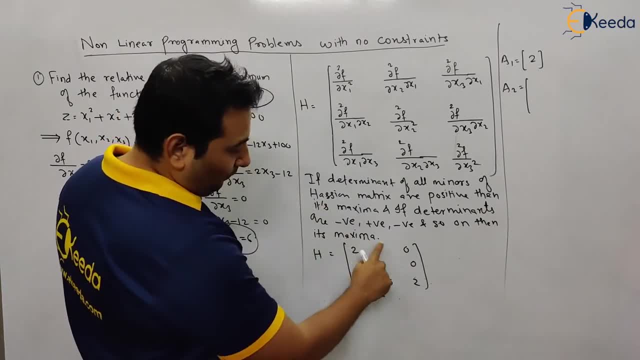 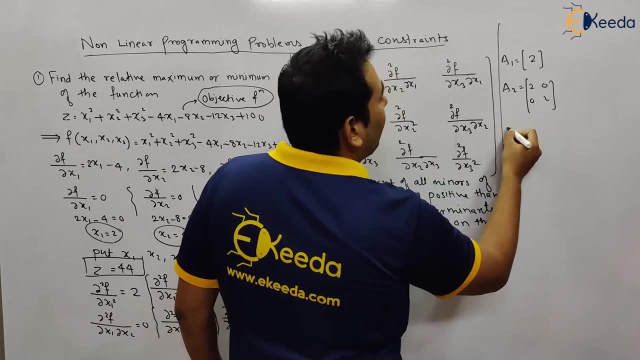 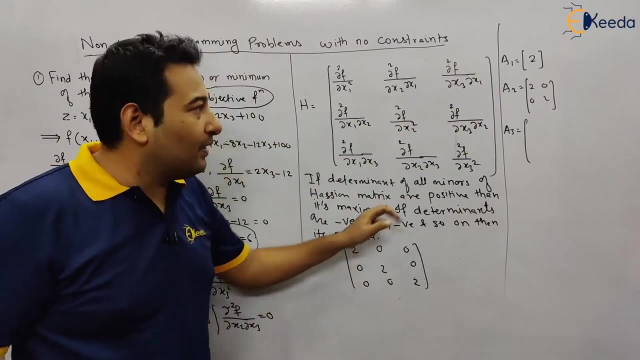 miner means two rows, two columns, but the, this, this for rows, and two columns, these four. so that is what to zero, zero, two. and a3 means the complete matrix. three cross 3, a1 means 1 cross 1, first row, first column. a2 means 2 cross 2 and a3 means 3. 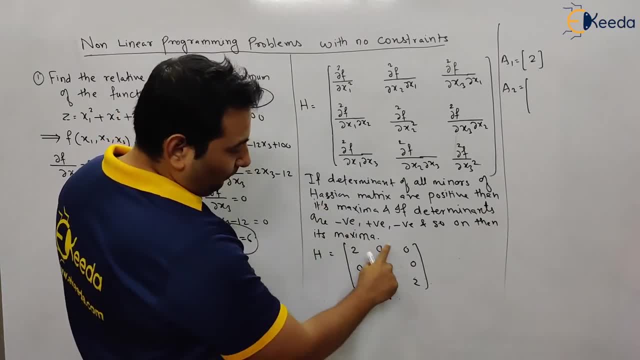 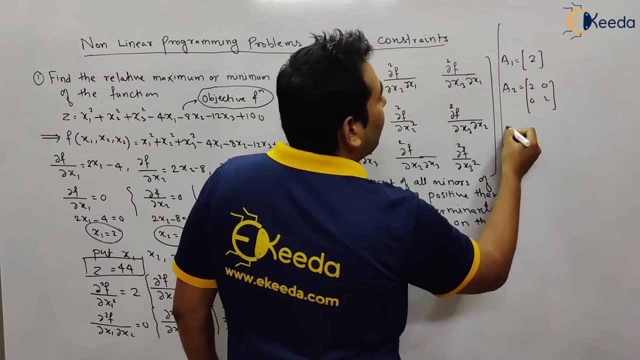 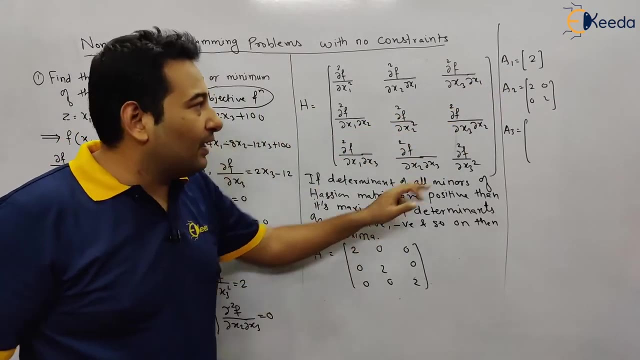 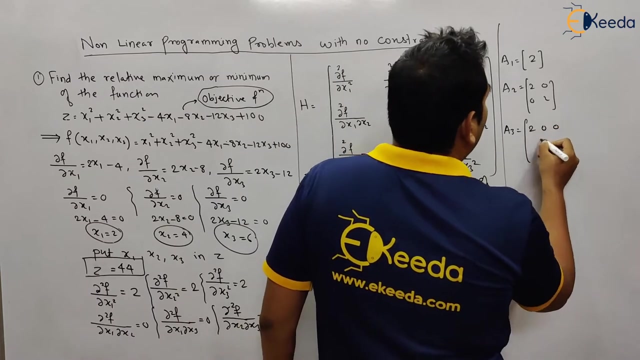 means two rows, two columns means these four: two rows and two columns, these four. so that is what 2002 and A3 means the complete matrix. 3 cross 3,. A1 means 1 cross 1, first row, first column. A2 means 2 cross 2 and A3 means 3 cross 3. that is your entire matrix. 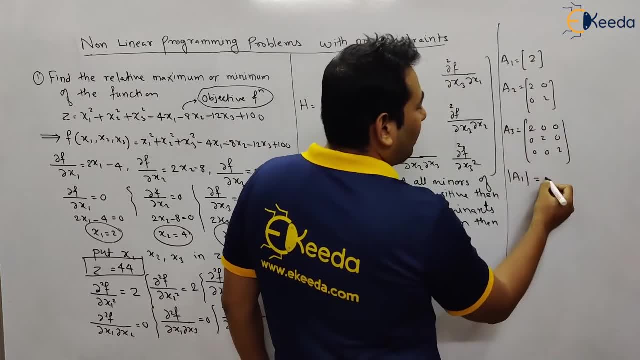 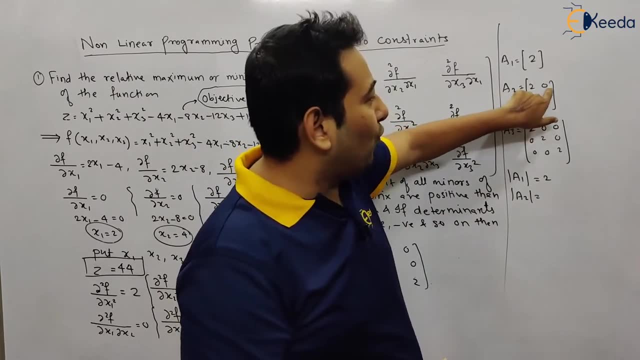 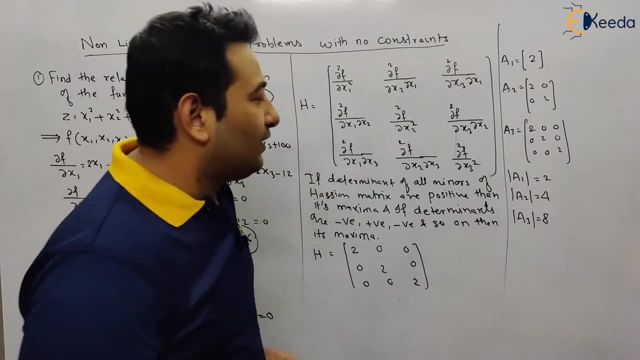 If you find the determinant, its determinant, there is only one element, that is, two determinant. determinant of this element: this matrix 2 to 4 minus 0, that is 4. and if you find determinant of the last, that is 8, see here all the determinant values are positive. see here if determinant. 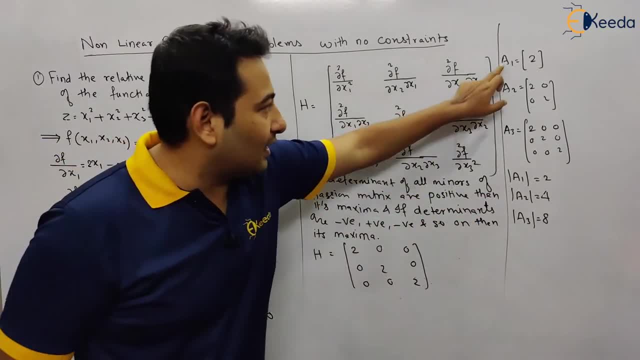 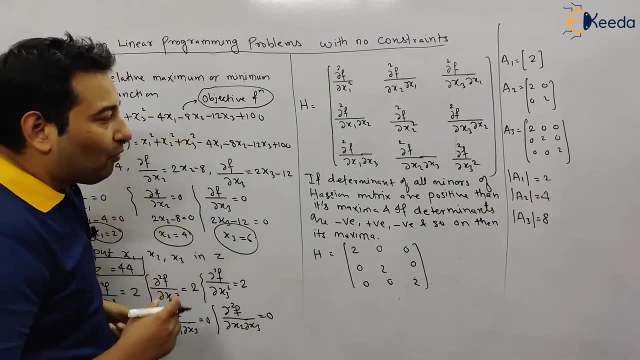 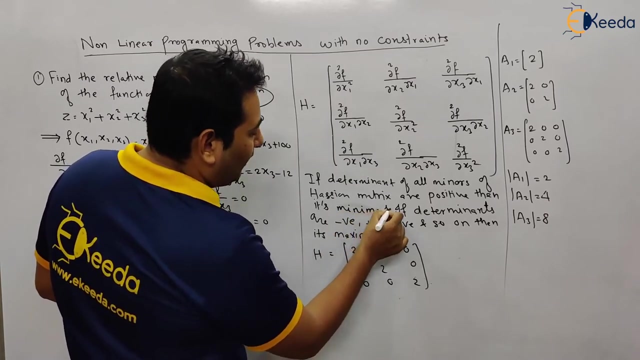 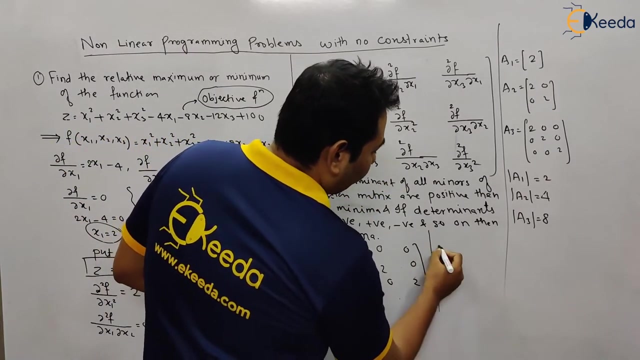 of all minors of Hessian matrix. these are the three minors. all are positive, see here, then its all are positive, then it is minima. all are positive, then it is a minima. and if determinants are negative, positive, then it is maxima. okay, since all the values are, since. 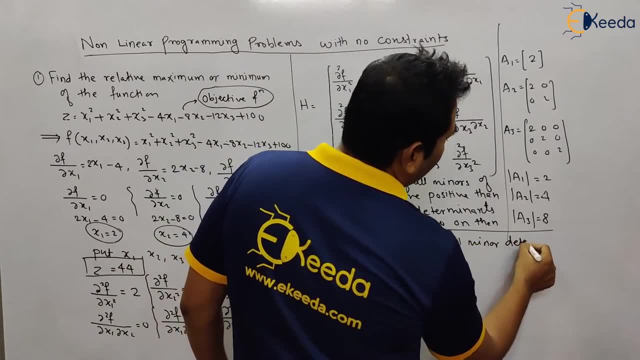 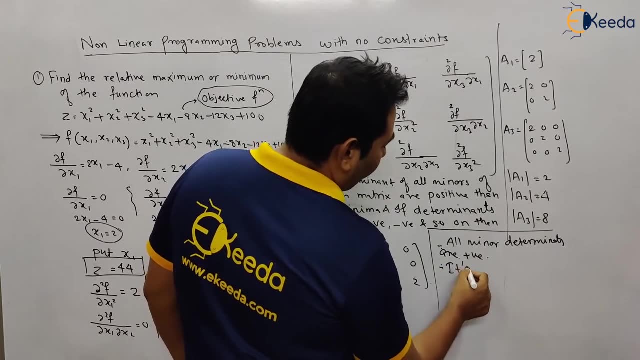 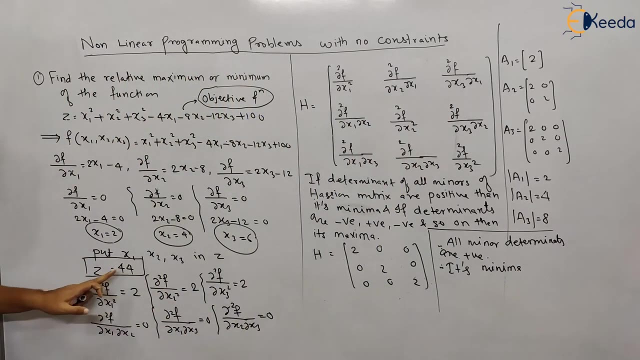 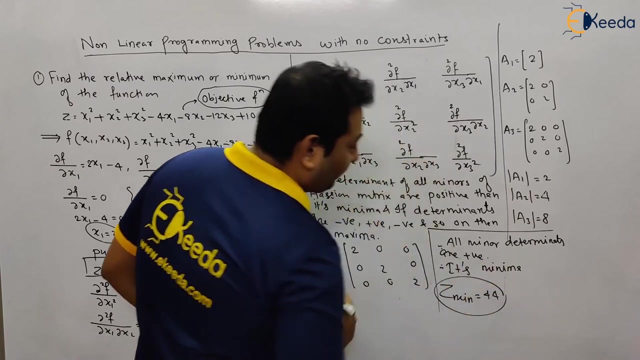 all minor determinants are positive. Therefore, therefore, it's minima and the solution that we got- see here, we already got this solution- that is, z is equal to 44. that is the minimum value of the function. so that is your required solution. so just to write this minima here we have to solve this, see once again, once again, let 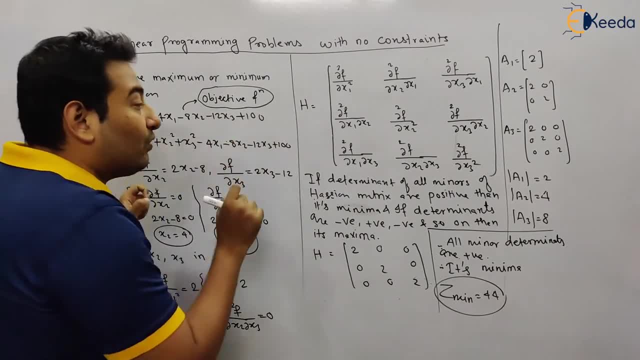 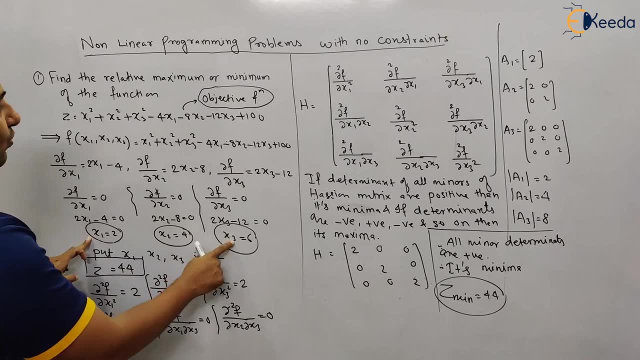 me summarize it quickly. this is my function and I need to find out the relative maxima or minima, and the solution is: z is equal to 44. that I got it by putting x1, x2, x3, x4,, x1, x2 and x3 here, so I got my solution here only. but I just need to check whether the 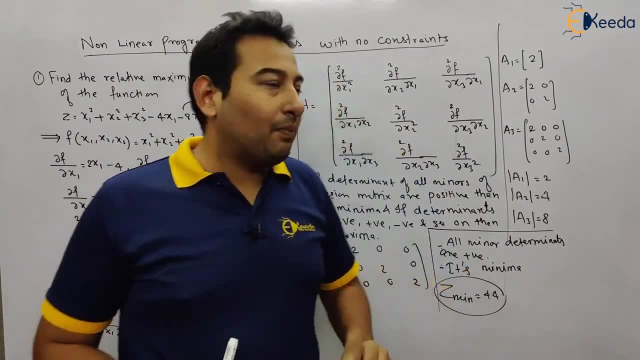 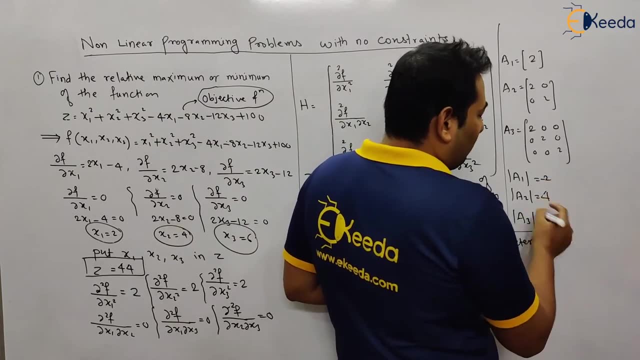 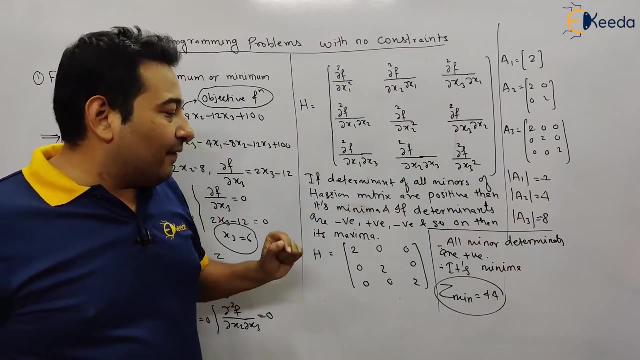 value that I got is a maxima or minima. for that purpose I need to go ahead with this particular procedure. suppose, after solving, suppose this value is minus, this is plus and suppose this is minus after solving the determinant, then it is negative, positive and negative. in that case the value that we got, z, will be maxima. that is written here. hope this is. 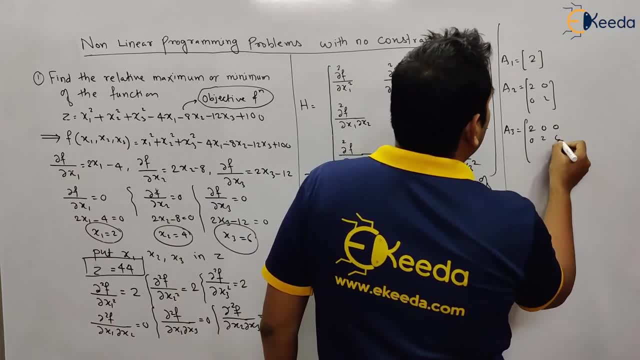 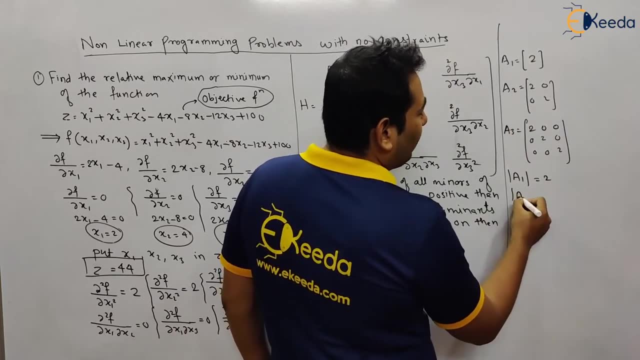 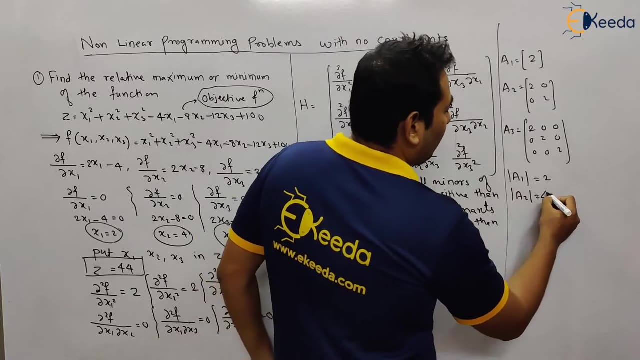 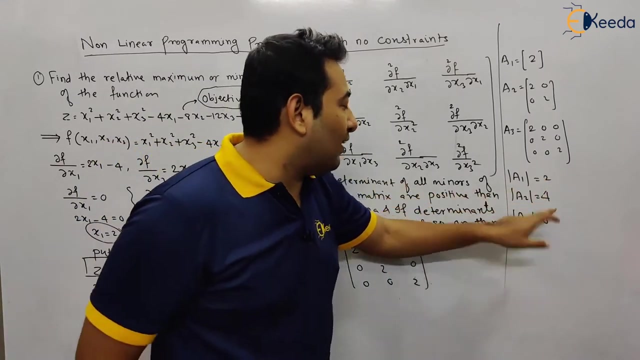 cross 3. that is your entire matrix. If you find the determinant, its determinant, there is only one element, that is 2. determinant determinant of this element, this matrix 2 to 4 minus 0, that is 4. and if you find determinant of the last, that is 8. see here all the determinant values are positive. see here if determinant. 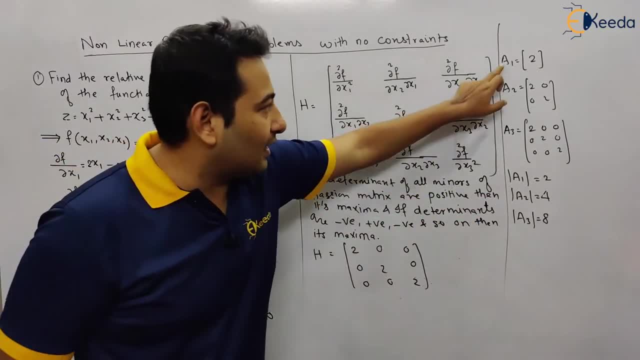 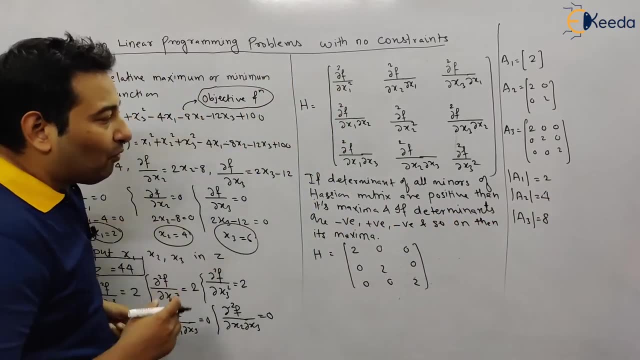 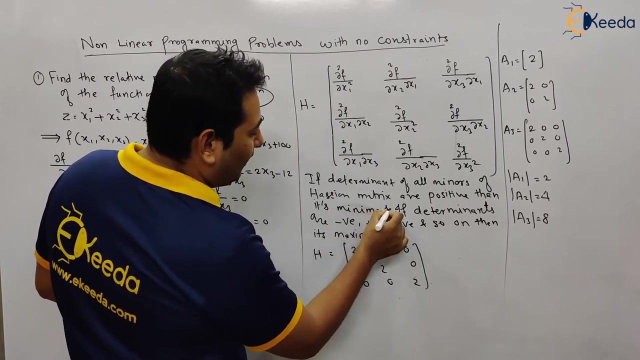 of all minors of hessian matrix. these are the three minors. all are positive, see here, then its all are positive, then it is minima. all are positive, then it is minima. and if determinants are negative, positive, then it is maxima. ok, Since all the values are positive. 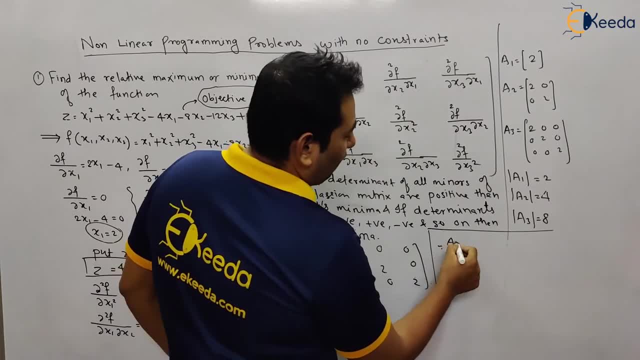 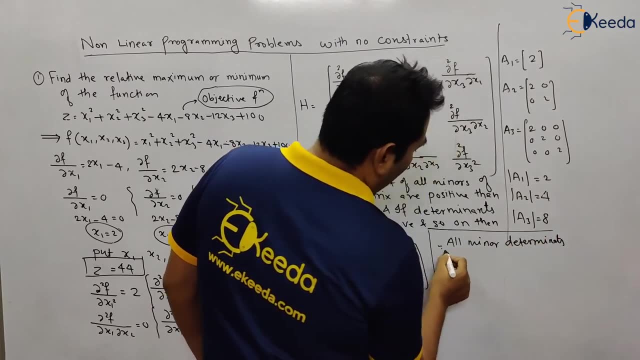 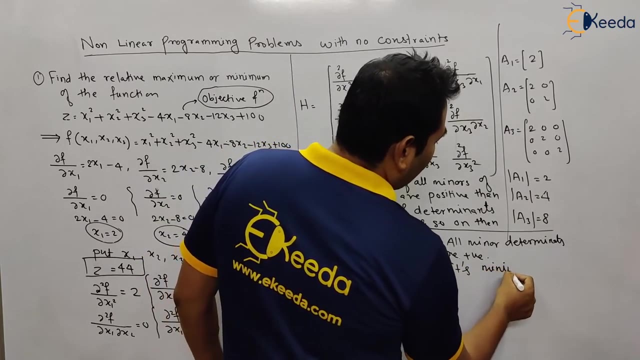 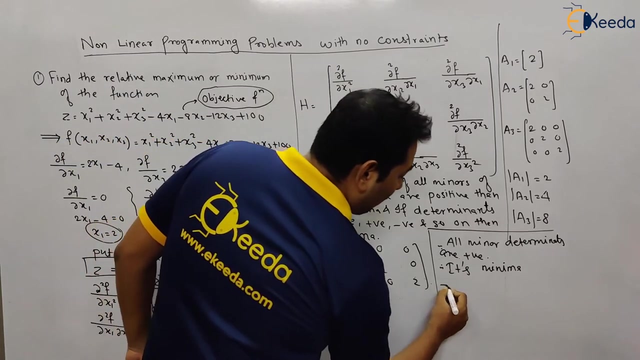 Since all minor determinants are positive. therefore its minima and the solution that we got- see here, we already got this solution- that is, z is equal to 44. that is the minimum value of the function. So that is your required solution. So just to write. 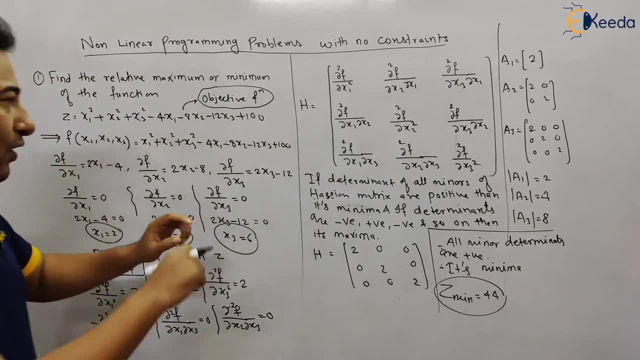 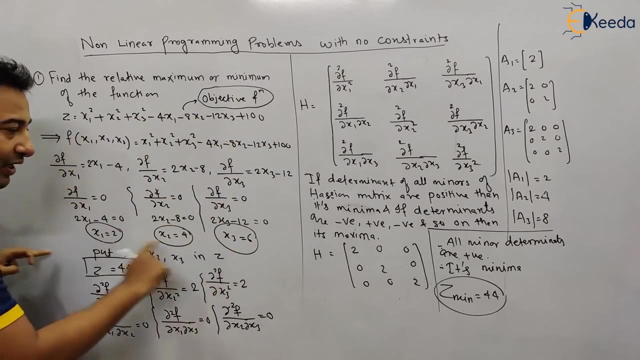 Write this minima here. we have to solve this. see once again. let me summarize it quickly. this is my function and I need to find out the relative maxima or minima, and the solution is: z is equal to 44. that I got it by putting x1, x2 and x3 here, so I got my solution here. 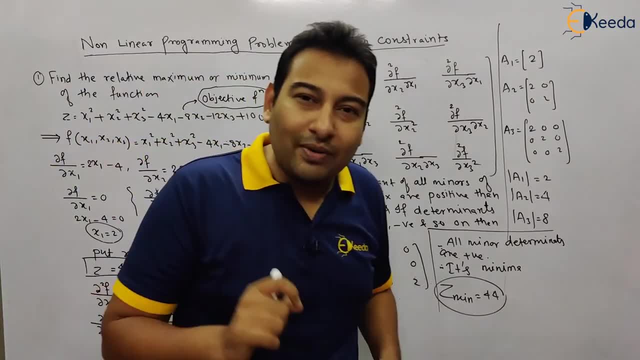 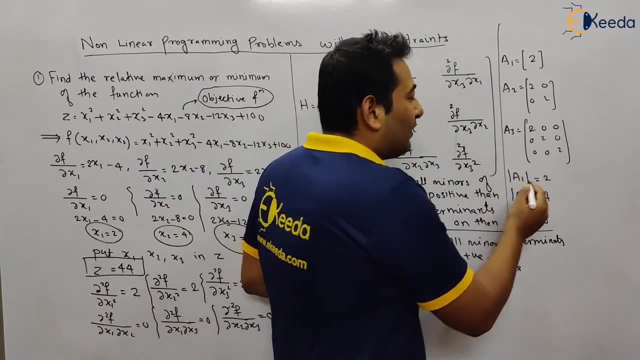 only, but I just need to check whether the value that I got is a maxima or minima. for that purpose, I need to go ahead with this particular procedure. suppose, after solving, suppose this value is minus, This is plus, And suppose this is minus after solving the determinant, then it is negative, positive and 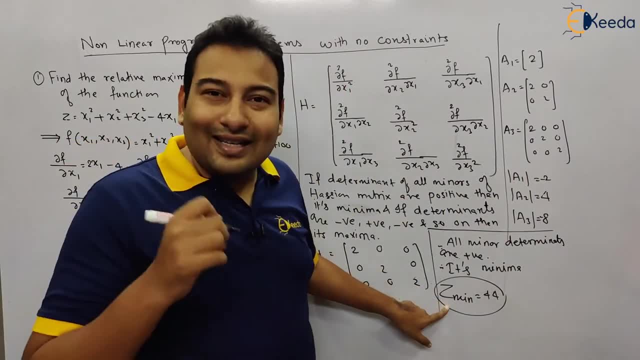 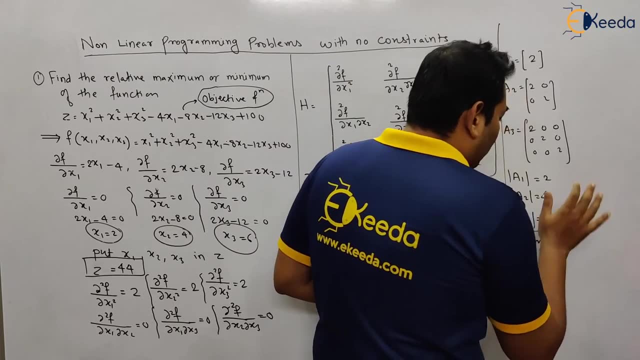 negative. in that case, the value that we got z will be maxima. that is written here. Hope this is clear. we done with the problem. please go through it. solve it properly. it will be very clear. Thank you.